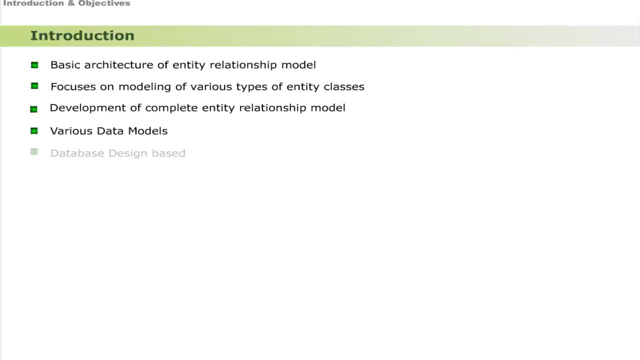 History of various data models and the current trends on which database design is based. It also focuses on the basic database design derived from entity relationship model Objectives. The objectives of the unit are to understand Architecture of entity relationship model, Various types of relationships, How the complexities of relationship are handled. 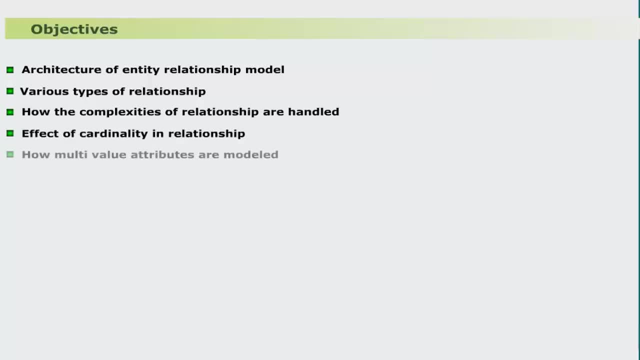 The effect of cardinality in relationships, How multi-valued attributes are modeled. How time-dependent attributes are modeled. How associative entity types are modeled. Hierarchical data model, Network data model, Relational data model. Why relational data model is in use and The basics of database design. The ER model. 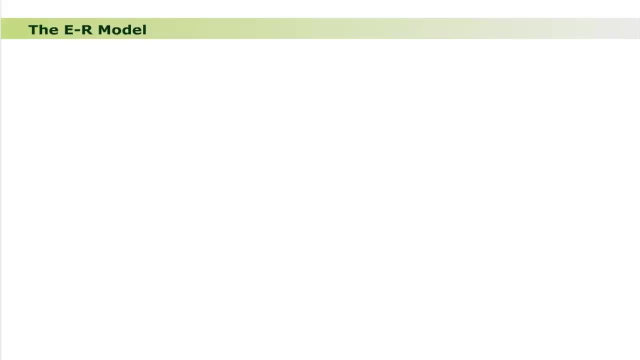 An entity relationship model, also called ER model, is a detailed logical representation of the data. It is expressed in terms of Entity classes in the business environment, the relationship or associations among those entity classes, along with their attributes. An ER model is normally expressed as an entity relationship diagram. 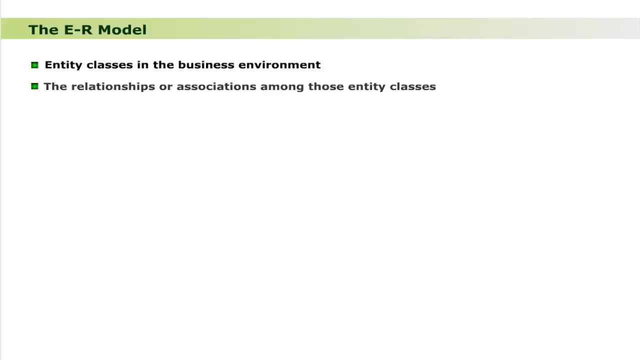 commonly referred as ER diagram, which is a graphical representation of an ER model- ER model notations. Let us now discuss the symbols which are used to develop the ER model. These are: Rectangle. The entity class is represented by a rectangle. The name of entity class is written inside. 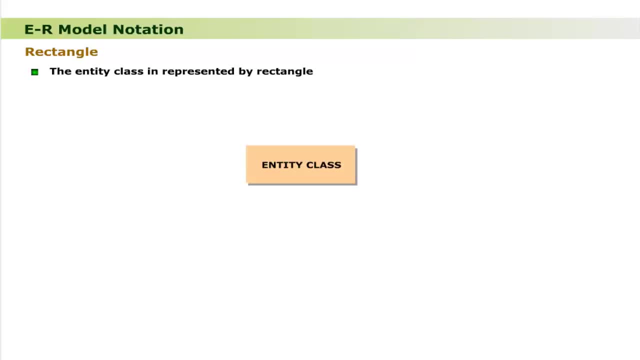 As shown. For example, The entity class student is represented As shown. Oval: The attributes are represented as an oval shaped symbol. The name of attribute is written inside, As shown, For example. The attribute name is represented As shown. Dear learners, Let us discuss the representation of different types of attribute. 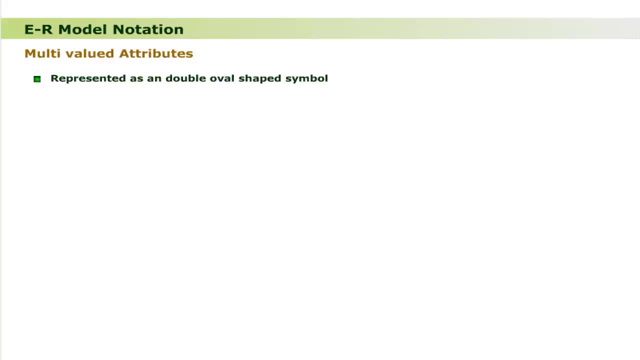 These are Multi-valued attribute. The multi-valued attribute is represented by double oval shaped symbol. The name of attribute is written inside As shown. For example, The multi-valued attribute courses are represented As shown. Derived attribute: The derived attribute is represented by dashed oval shaped symbol. 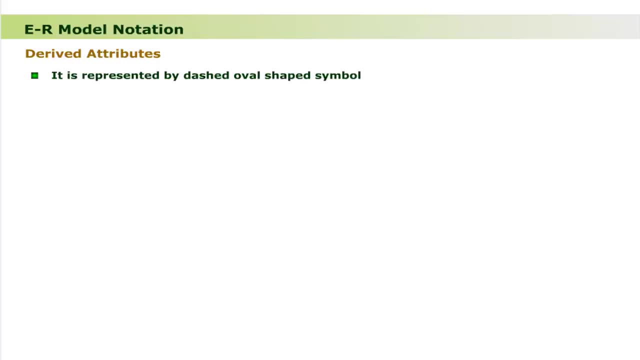 The name of attribute is written inside As shown, For example. The derived attribute- age- is represented As shown. Primary key attribute. The primary key attribute is represented as an oval shaped symbol. The name of attribute is underlined and written inside As shown, For example. 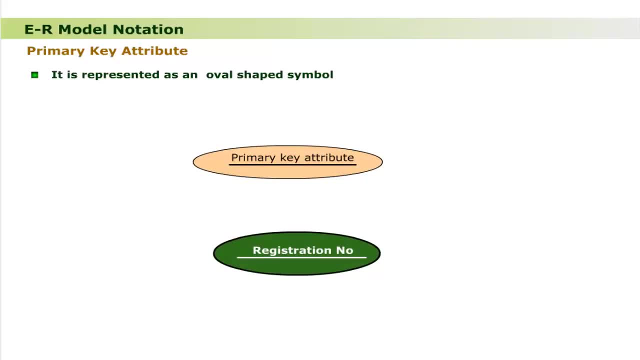 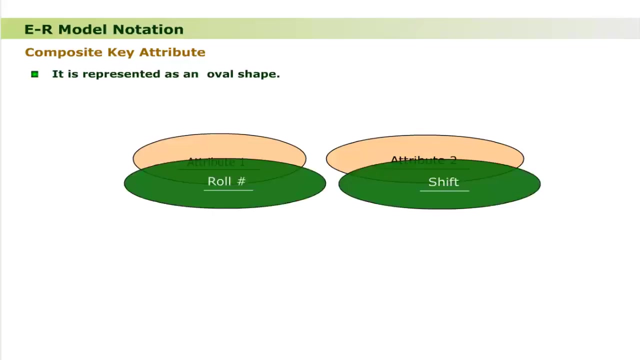 The attribute registration number is represented As shown. Composite key attribute. Each attribute of composite key is represented by an oval shaped symbol With underlying the attribute name written inside, As shown. For example, The attributes roll number and shift are shown as composite key. The ER model. 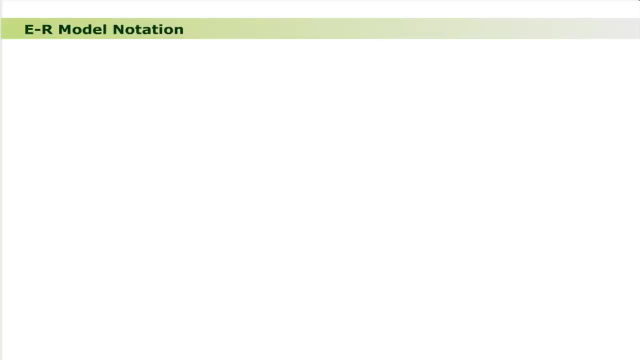 An entity relationship model, also called ER model, is a detailed logical representation of the data. It is expressed in terms of Entity classes in the business environment, the relationship or associations among those entity classes, along with their attributes. An ER model is normally expressed as an entity relationship diagram, commonly referred as ER diagram, which is a graphical representation of an ER model. 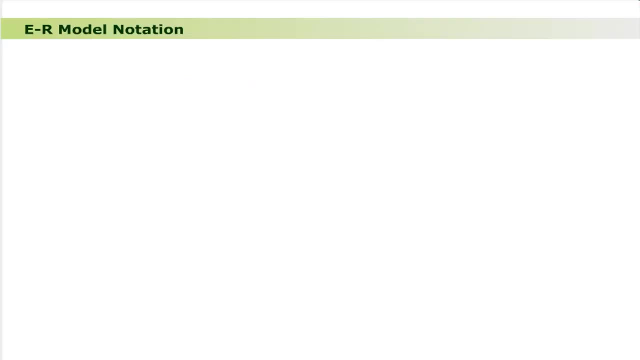 ER model notations. Let us now discuss the symbols which are used to develop the ER model. These are: Rectangle: The entity class is represented by a rectangle. The name of entity class is written inside. As shown, For example, The entity class student is represented. 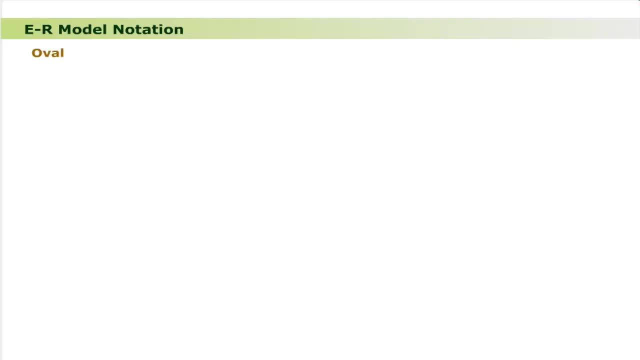 As shown. Oval- The attributes are represented as an oval shaped symbol. The name of attribute is written inside, As shown. For example, The attribute name is represented As shown. Dear learners, let us discuss the representation of different types of attribute. These are Multi-valued attribute. 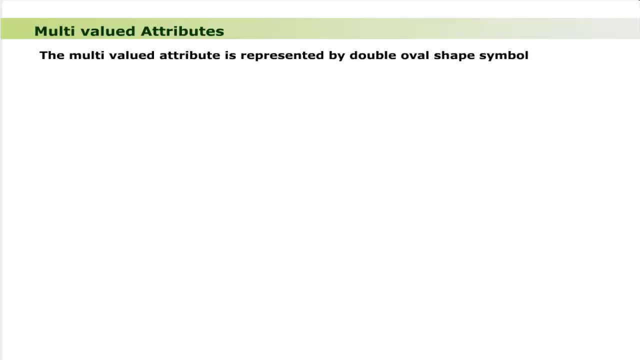 The multi-valued attribute is represented by double oval shaped symbol. The name of attribute is written inside As shown. For example, The multi-valued attribute courses are represented As shown. Derived attribute. The derived attribute is represented by dashed oval shaped symbol. The name of attribute is written inside. 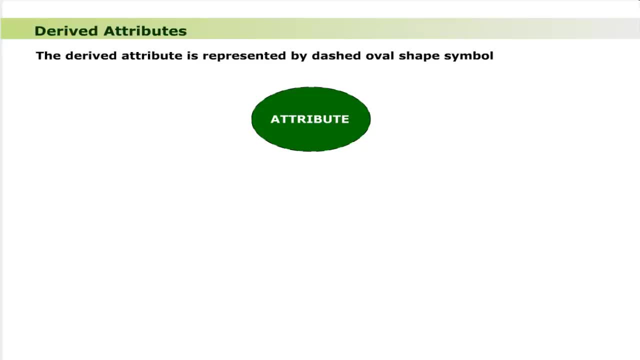 As shown. For example, The derived attribute age is represented As shown. Primary key attribute. The primary key attribute is represented as an oval shaped symbol. The name of attribute is underlined and written inside As shown. For example, The attribute registration number is represented As shown. 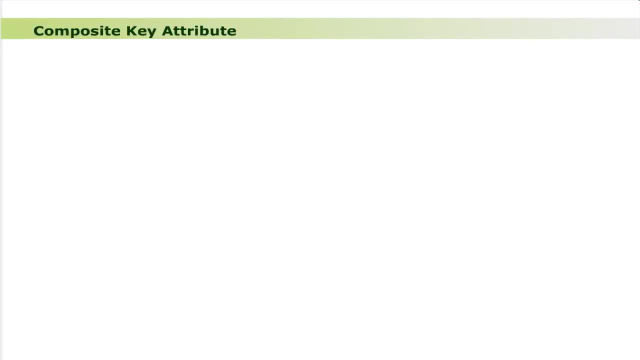 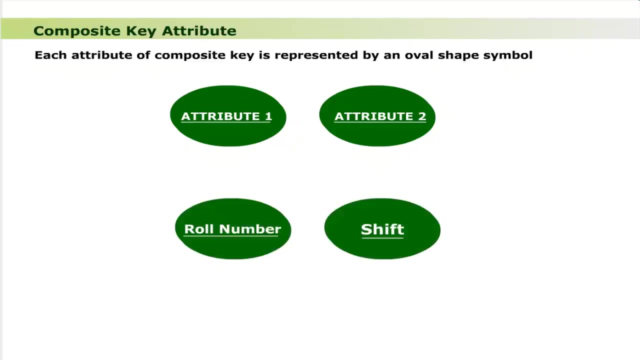 Composite key attribute. Each attribute of composite key is represented by an oval shaped symbol With underlying the attribute name written inside, As shown. For example, The attribute's roll number and shift are shown as composite key. Dear learners, After types of attribute representation, the next symbol of ER model is: 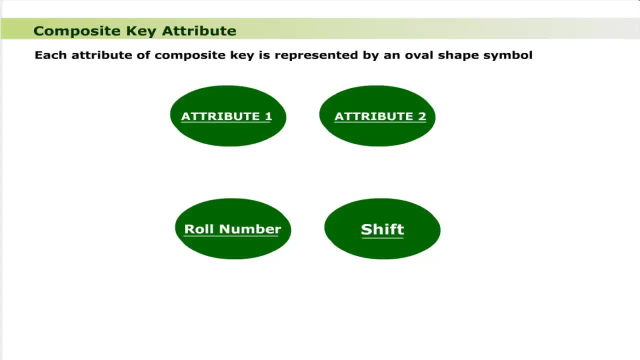 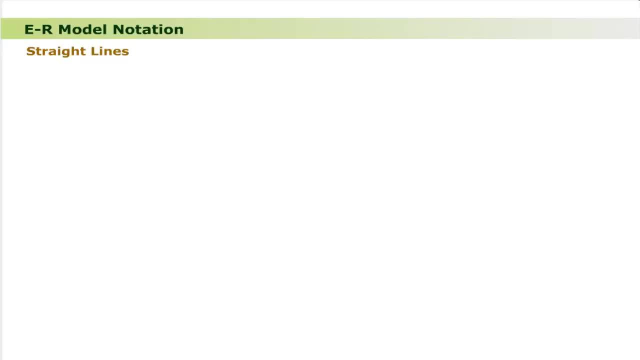 Straight lines. The next symbol of ER model is Straight lines. Recall: We learned previously that attributes are the defined properties of an entity class. This means that attributes are always associated with an entity class. The straight lines are used to connect attributes to an entity class. 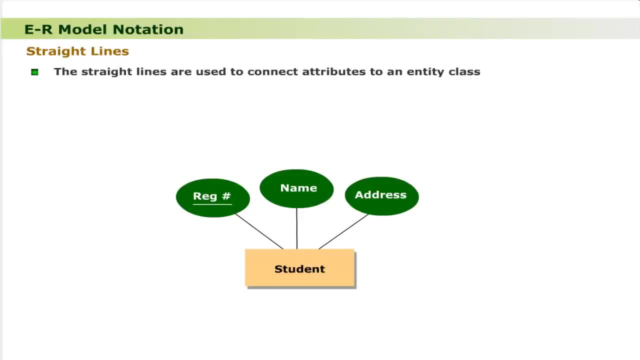 As shown. For example, The entity class student has three attributes: Registration number, name and address. These are connected by straight lines. As shown. Diamond ıl. The ratio of two properties is dipole, The ratio of twoaaS to inboard classes asCom块. This is what is called as diamond. 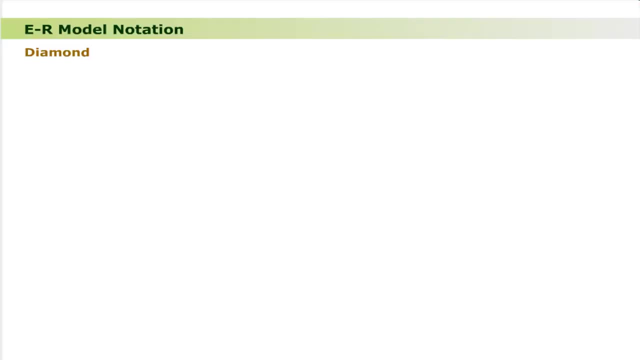 Google For the Case. If There are Listed Every Terre, There are сч star b, For example. the relationship named register is represented as shown. Now it is time to show a simple example of ER model. Consider the statement: A student is allowed to register a project in the final semester. 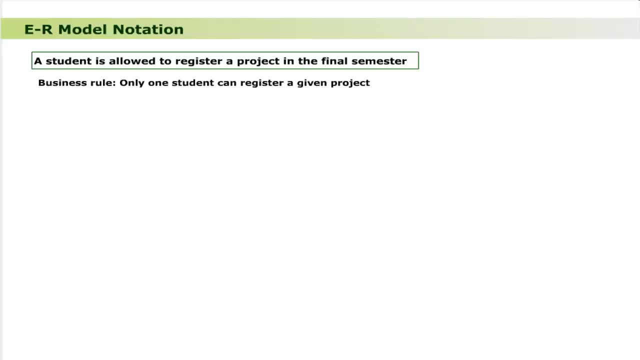 The business rule is only one student can register a given project. There are two entity classes. These are: student- Let the attributes are registration number, which is the primary key, and name Project. Let the attributes are code, which is the primary key, and title. 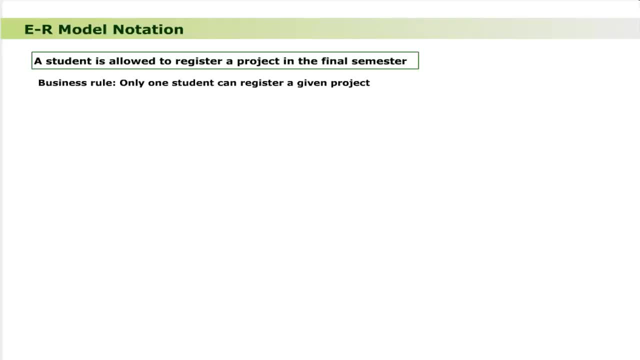 This situation can be represented in ER model as shown. The relationship register acts as glue through straight lines to connect entity class, student with attributes, registration number and name. another entity class, project with attributes, code and title. Dear learners, the type of association changes in ER model. 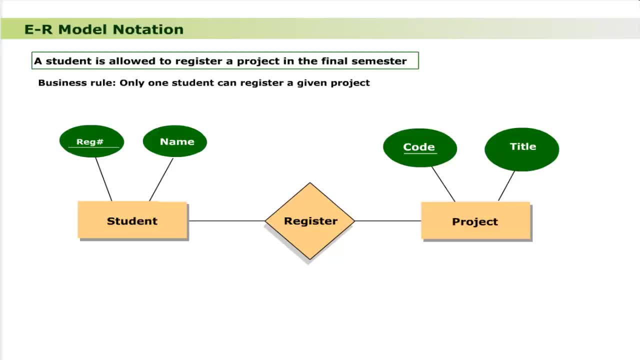 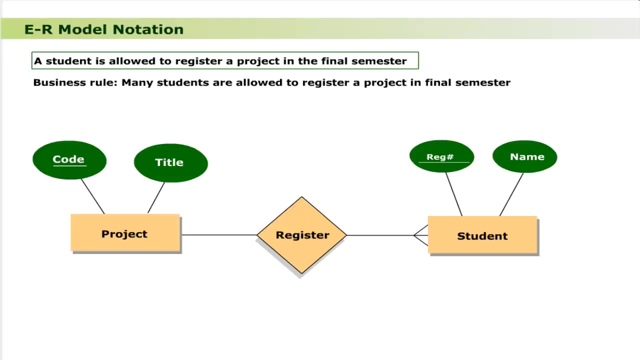 If the business rules are changed. This is discussed here. Let us change the business rule for the problem stated just before that many students are allowed to register a given project in the final semester. This situation is represented in ER model as shown. The type of association is changed to one to many. 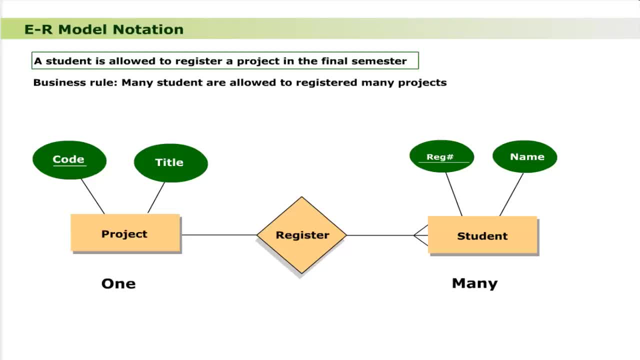 Now let us change the business rule once again, As many students are allowed to register many projects in the final semester. This situation is represented in ER model, as shown. This time, the type of association is changed to many, to many. This time, the type of association is changed to many, to many. 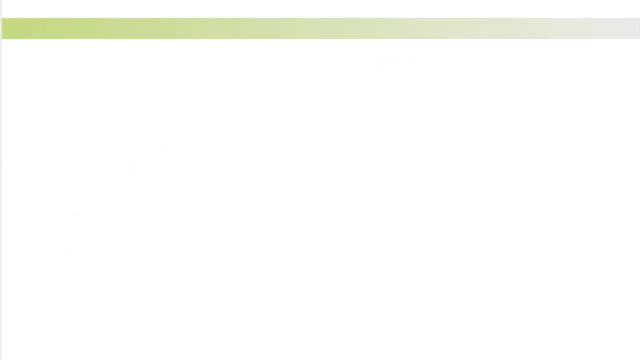 This time the type of association is changed to many, to many Types of relationship. Dear learners, the relationship discussed previously takes many forms, which are discussed here. United relationship: It is relationship between instances of same entity class. It means that only one entity class is associated with a given relationship. 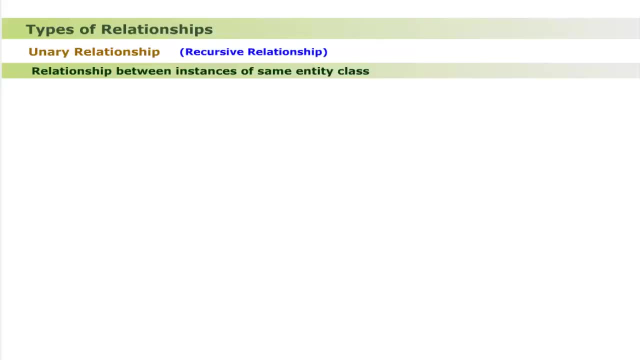 The unitary relationship is also called recursive relationship. The general representation in ER model is shown as, For example, one employee that is manager manages another employee that is staff or worker. The manager and staff or worker both belong to employee entity class. There is a relationship named manage. 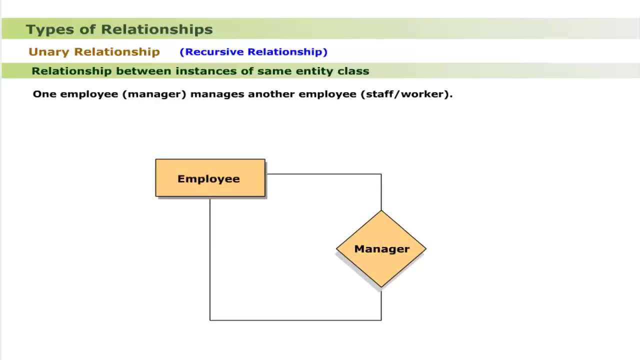 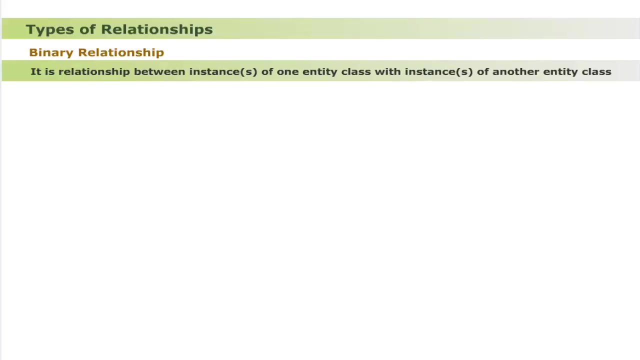 The ER model is shown as It shows that one instance of entity class employee, that is, manager, manages another instance of same entity class. that is staff Binary relationship. It is relationship between instances of one entity class with instances of another entity class. It means that two entity classes are involved in a given binary relationship. 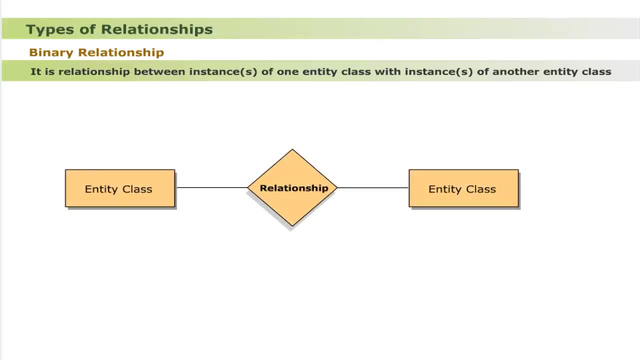 It is represented in ER model as, For example, a customer places an order. There are two entity classes: customer and order. There is a named relationship place. The ER model is shown as The relationship place connects logically the entity class customer with entity class order. 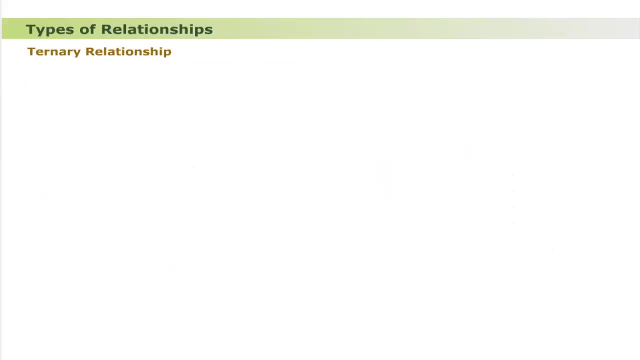 Ternary relationship. It is relationship between instances of three entity classes with one another. It means that three entity classes are involved in a given ternary relationship. It is represented in ER model, as shown, For example, many students registered many courses and many faculty members teach many. 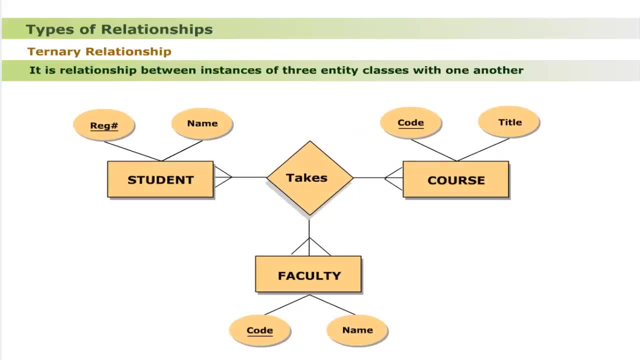 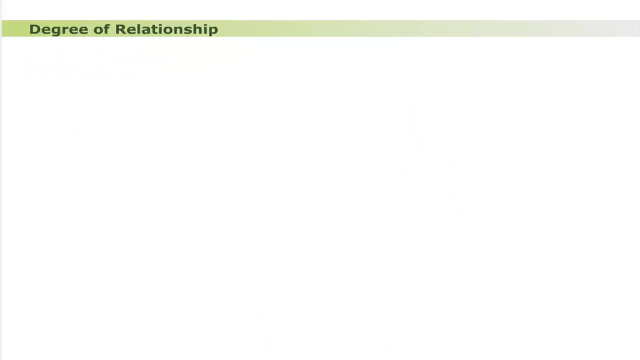 courses, The ER model is shown, as In this model the relationship takes connect logically three entity classes: student, course and faculty member. Dear Learners, The number of entity classes for a given relationship is not restricted to three, but rather any number of entity classes can be used to determine the degree of relationship. 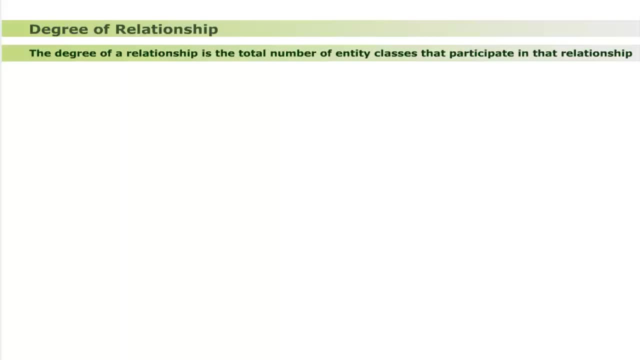 The degree of a relationship is the total number of entity classes that participate in that relationship. Dear Learners, Look at these examples. Example number 1: The relationship managed has only one entity class, that is employee. Therefore, the degree of relationship managed is one. 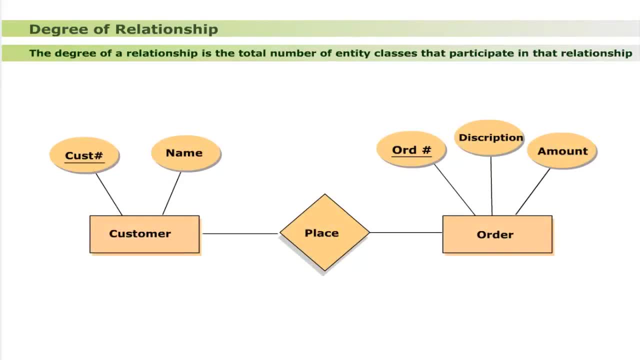 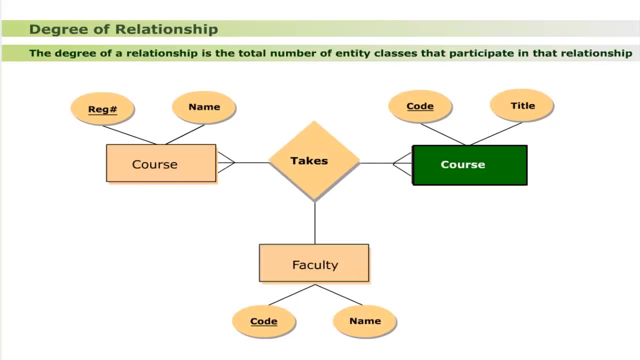 Example number 2: The relationship place has two entity classes that are customer and order. Therefore, the degree of relationship place is two. Example number 3: The relationship takes has three entity classes that are student, faculty and course. Therefore, the degree of relationship takes is three. 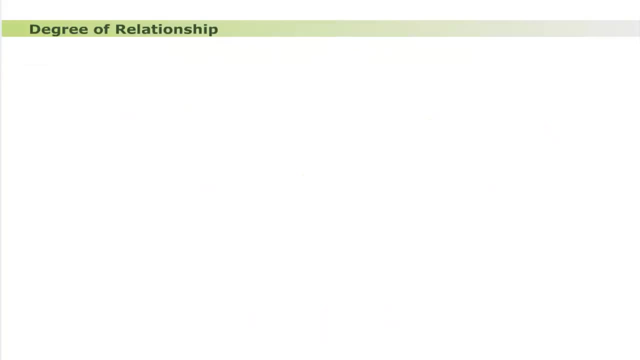 Dear Learners, The degree of a relationship is not restricted to three, but the degree of a relationship beyond ternary is considered being a poor practice as it increases complexity. Therefore, the higher degree relationship are advised to decompose in order to make it simple. 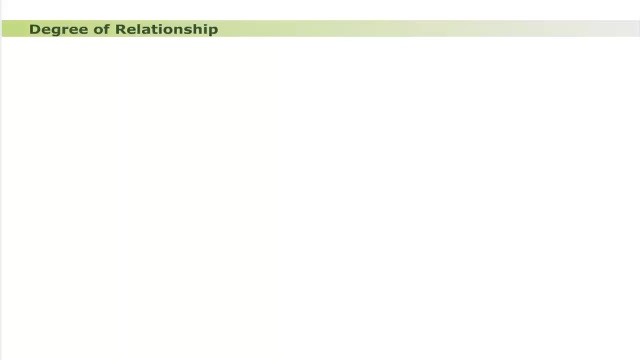 Example number 4: Let us now discuss how the higher degree relationship create complexity by taking this example. as shown, Look at the ER model. The degree of relationship takes is four. There are four entity classes involved. These are: 1. Student, 2. 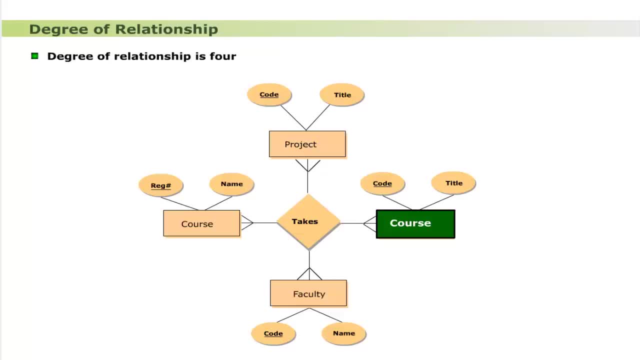 Faculty, 3. Project, 4. Course. The complexity can be easily judged by reading the model, as Many students registered many courses. Many students registered for many projects. Many faculty members are assigned many courses. Many faculty members supervise many projects. The single relationship is sometimes difficult to name. 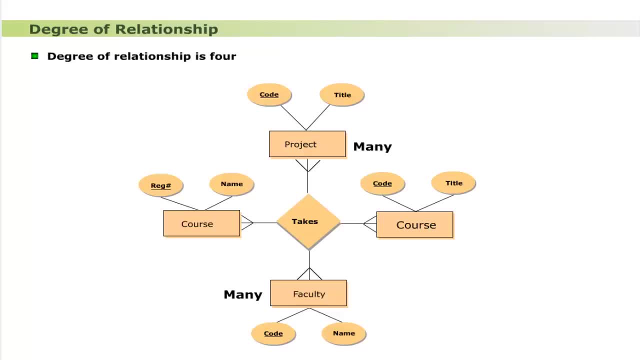 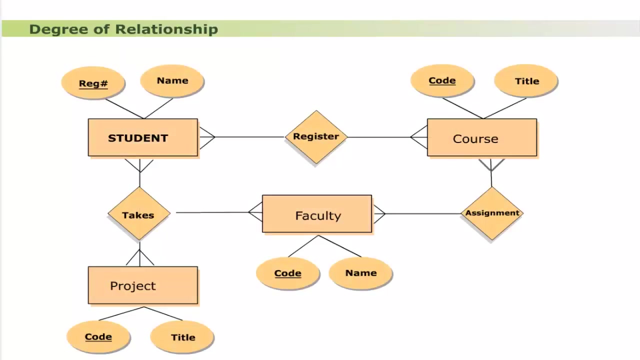 Moreover, the relationship takes shows a direct relationship between entity classes, project and courses which does not exist actually. The relationship takes may be decomposed as shown. Look at the modified version of degree 4: relationship takes. The relationship register connects entity class student with entity class course and. 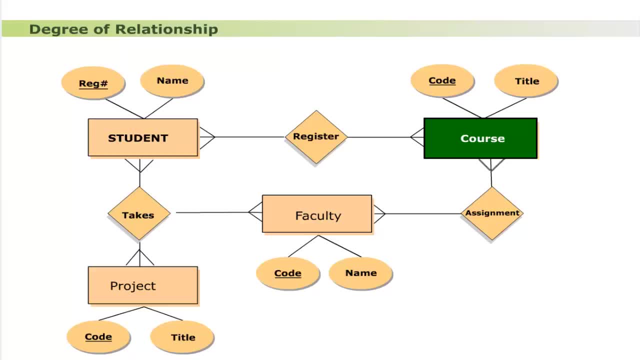 entity class course course, as many students register many courses. the relationship takes connects three entity classes: student, project and faculty, as many students register many projects and projects are taken by many faculty members. the relationship assignment connects entity class course with entity class faculty, as many courses are assigned to many faculty members. cardinality- cardinality is the 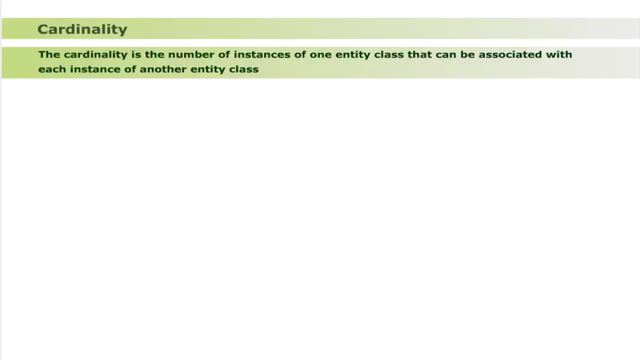 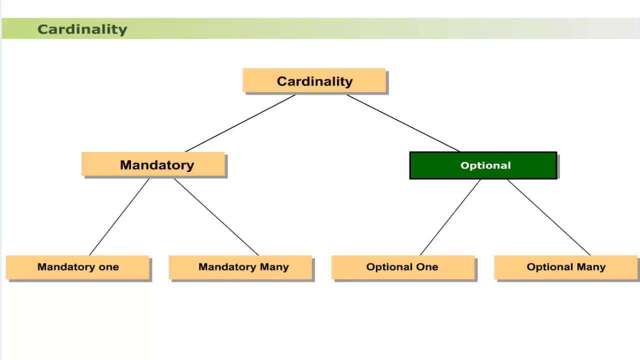 number of instances of one entity class that could associated with each instance of another entity class. let us now discuss cardinality in more detail by discussing various types of cardinality. these are mandatory cardinality and optional cardinality. the mandatory cardinality is further divided into mandatory one and mandatory many. similarly, the optional cardinality is 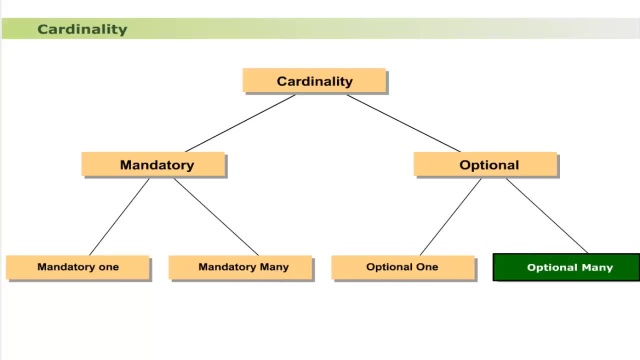 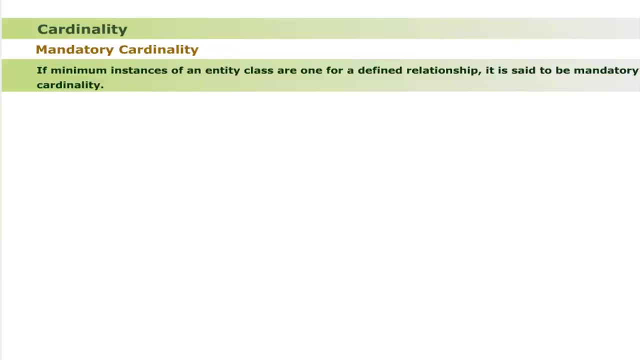 also further divided into optional one and optional many. let us now discuss each one in detail. mandatory cardinality: if minimum instances of an entity class are one for a defined relationship, it is said to be a mandatory cardinality. for example, a student must register minimum of one course in a semester. the cardinality of entity class course is: 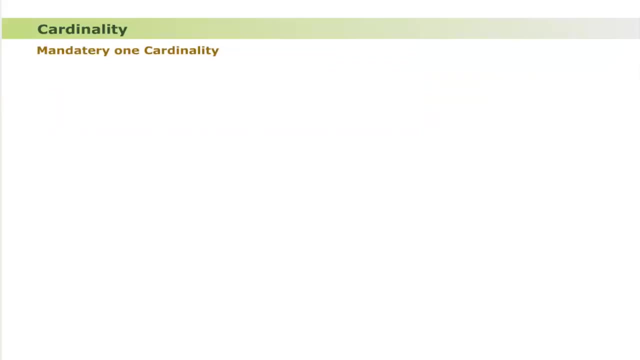 said to be mandatory, mandatory one: cardinality. the mandatory cardinality is said to be mandatory one if both minimum and maximum instances are one in a relationship. the general form of mandatory cardinality is shown as, for example, consider a statement that a student must take a project in the 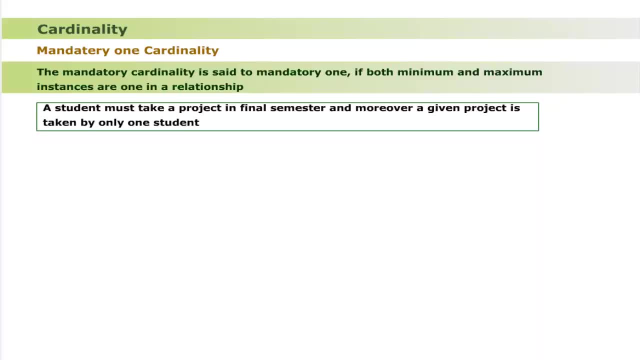 final semester and, moreover, a given project is taken by only one student. look at the ER model. as shown, the cardinality of entity class student is mandatory one, as the minimum and maximum value of a student is one in the relationship takes. Similarly, the cardinality of entity class project is: 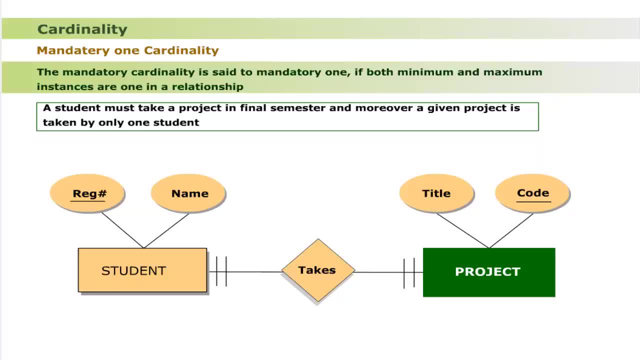 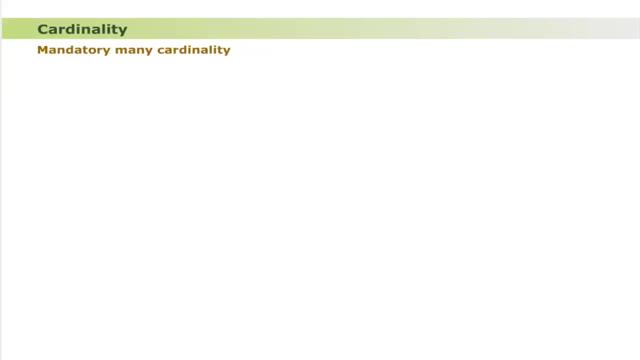 mandatory one as the minimum and maximum value of a project is one in the relationship takes Mandatory Many Cardinality. The mandatory cardinality is said to be mandatory many if minimum instance is one and maximum instances are more than one in a relationship. The general form of mandatory cardinality is shown as, for example: consider a statement: 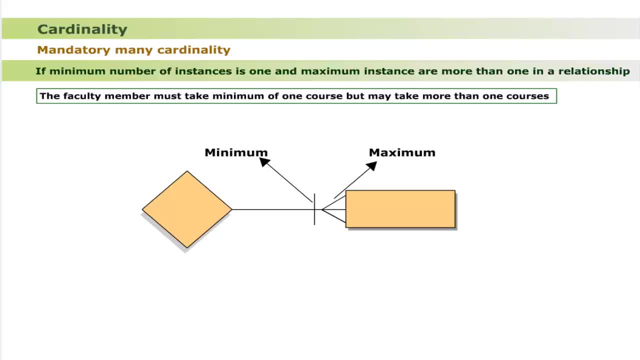 that a faculty member must take minimum of one course but may take more than one courses. Moreover, a given course is taken by only one faculty member. Look at the ER model. as shown, The cardinality of entity class course is mandatory many as the minimum course value is one and maximum course value is many. in the relationship, 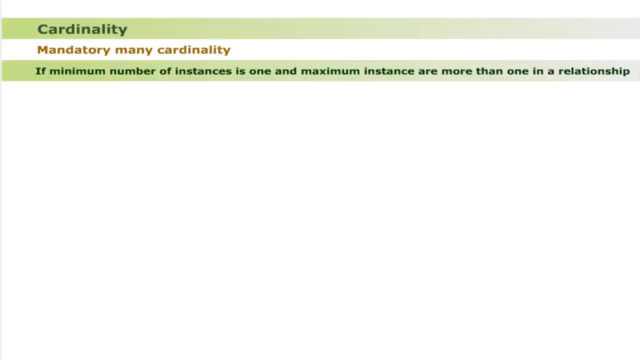 Teach, Dear learners, the many in mandatory many. cardinality may be a defined number, that is, 3.. It is represented as shown where n is any positive integer greater than 1.. Dear learners, let us now discuss optional cardinality in detail. 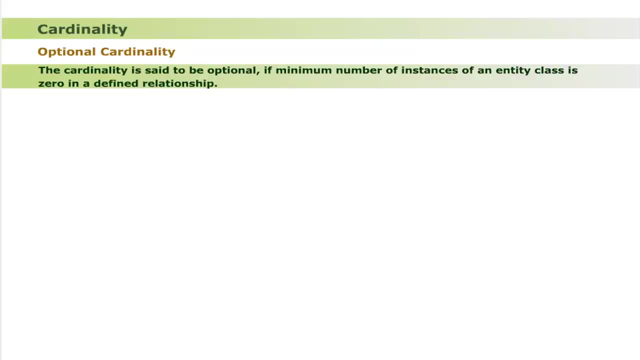 The cardinality is said to be optional if minimum number of instances of an entity class is zero in a defined relationship. For example, a faculty member may not take any course in a semester. Thus the cardinality of entity class faculty member is optional. Let us now discuss its types. 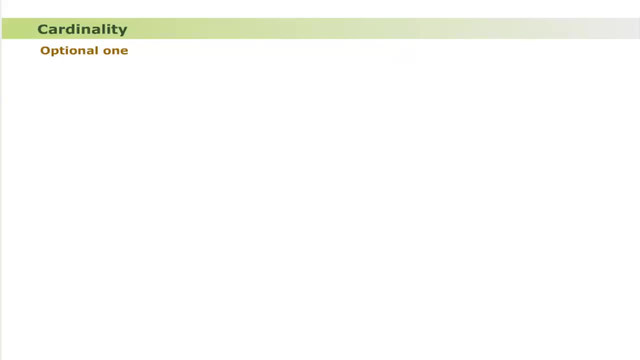 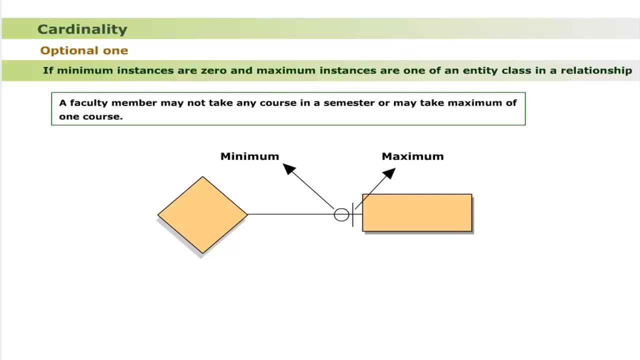 Optional 1. The optional cardinality is said to be optional 1 if minimum instances are zero and maximum instances are one of an entity class in a relationship. The general form of optional 1 cardinality is shown as, for example: consider a statement that a faculty member may not take any course. 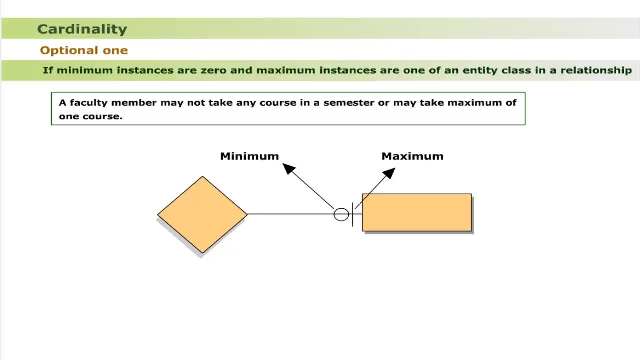 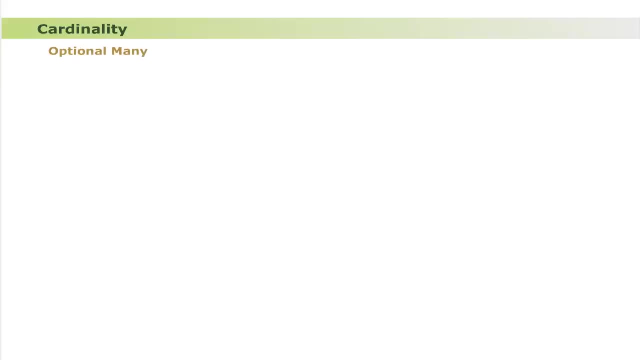 in a semester or may take maximum of one course. Look at the ER model. as shown, The cardinality of entity class course is optional 1 as the minimum course value is zero and maximum course value is one. in the relationship, take Optional many. The optional cardinality is said to be optional. 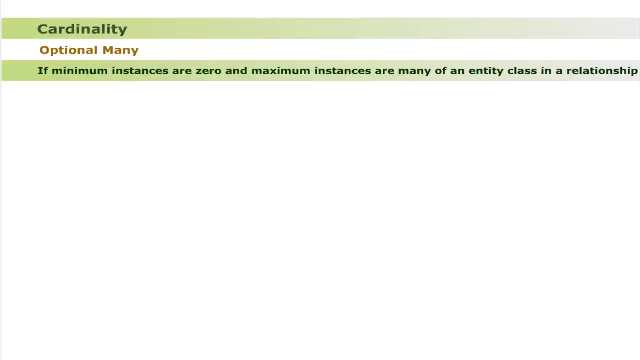 many if minimum instances are zero and maximum instances are many of an entity class in a relationship. The general form of optional many cardinality is shown as, for example, consider a statement that a faculty member may not take any course in a semester or may take many courses. 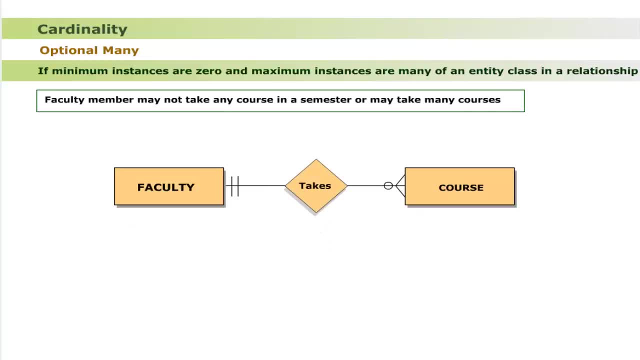 Look at the ER model as shown, The cardinality of entity class course is optional. many as the minimum course value is zero and maximum course value is many in the relationship. take Modelling Multi-Valued Attributes. Dear learners, let us consider an example of 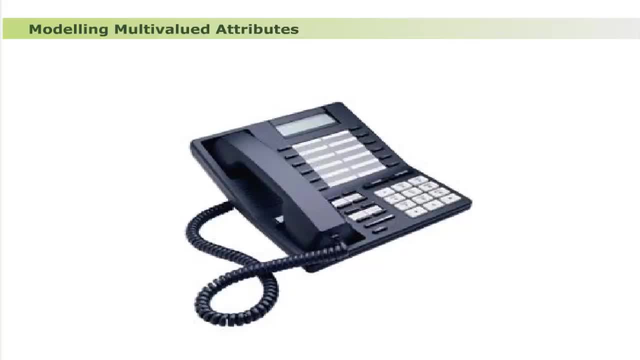 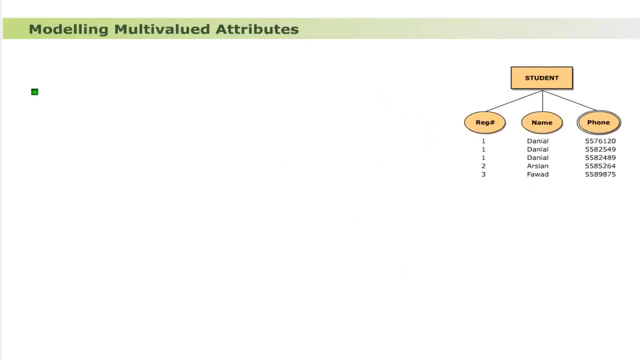 a multi-valued attribute phone before its modelling, as shown. as The analysis shows these drawbacks: 1. The attribute registration number is supposed to be a primary key, but due to existence of multi-valued attribute phone, it could not be defined. 2. There is redundancy due to existence of 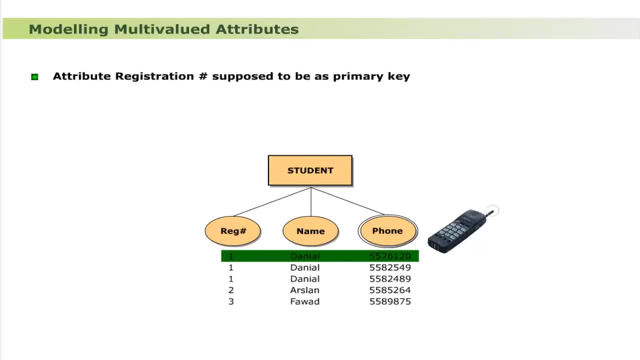 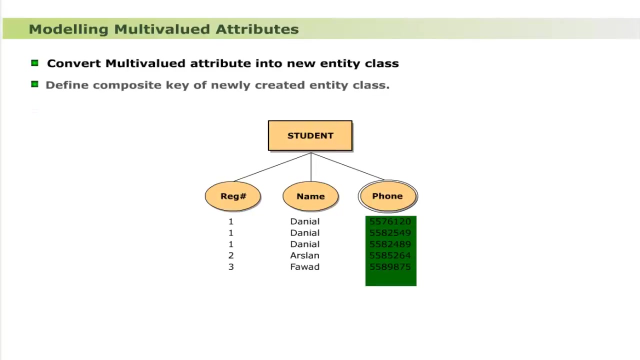 multi-valued attribute phone ie name- is placed three times because having three phone numbers, Thus adding value of phone number, creates redundancy, which is considered one of the major drawback. These problems can be resolved by adopting this general procedure. The multi-valued attribute is converted into new entity class. 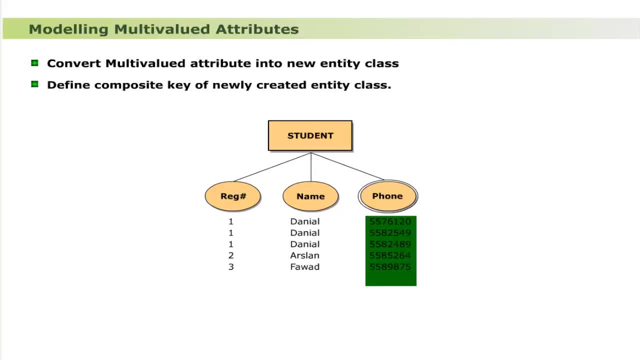 The newly created entity class have the composite key with primary key attribute of original entity class. Establish relationship between original entity class and newly created entity class class. Dear learners, there are two possibilities for existence of multi-valued attributes. Each one is dealt in a different way. 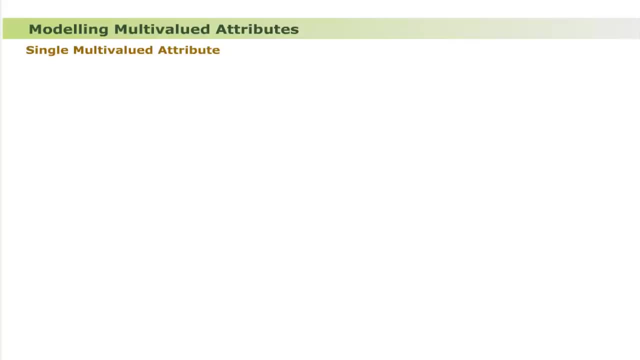 These are single multi-valued attribute. If there is only one multi-valued attribute in an entity class, then it is converted into separate new entity class. The class name and attributes are required to be defined. For example, consider the entity class student with two single-valued attributes: registration. 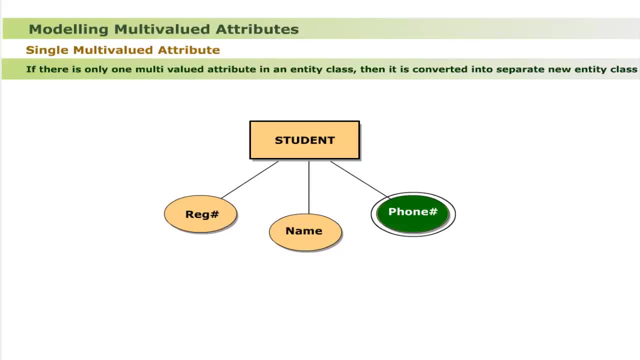 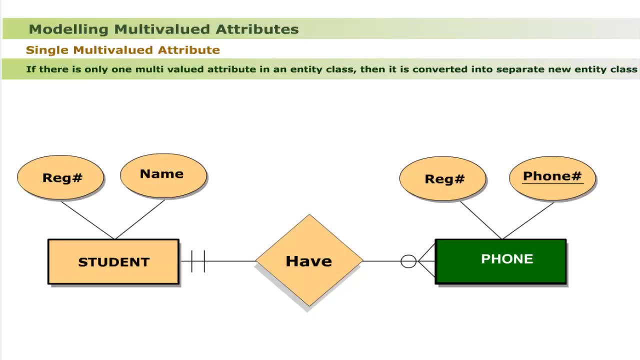 number and name and one multi-valued attribute phone. as shown, The multi-valued attribute phone number is converted into new entity class phone. as shown, The newly created entity class phone has two attributes: registration number and phone number. Both attributes collectively form composite key. 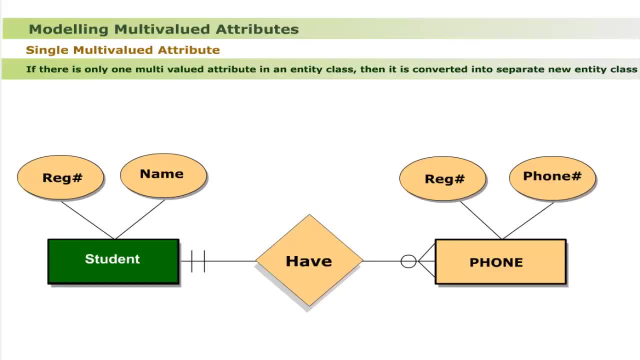 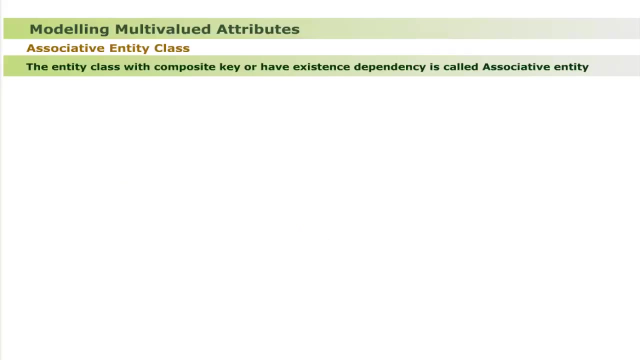 The relationship have is established between original entity class student and newly created entity class phone. Dear learners, this modeling of multi-valued attribute introduces new types of entity classes. These are associative entity class. The entity class with composite key or have existence dependency is called associative. 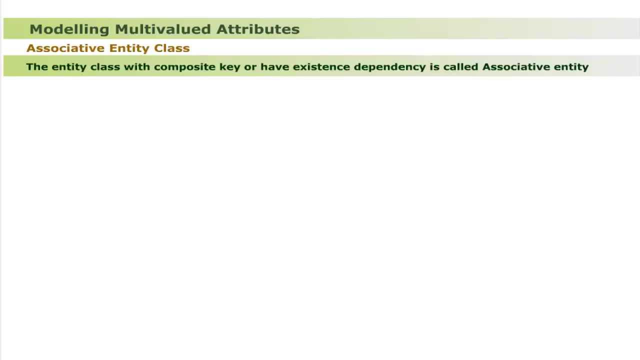 entity. The associative entity class is also called weak entity class. It is represented by a rectangle with lines. Regular entity class: The entity class with the primary key, or on which associative entity class is dependent, is called regular entity class. as shown, Dear learners, let us now discuss how many multi-valued attributes are dealt. 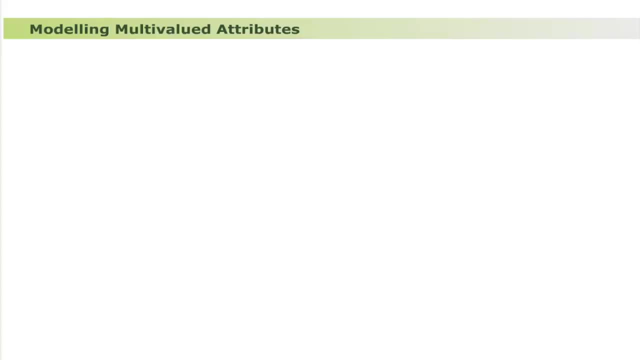 There are two possibilities for existence of many multi-valued attributes in an entity class. Let us now discuss each in detail. Logically related multi-valued attributes. Many multi-valued attributes are related to a class. Many multi-valued attributes that are logically related with one another form a group called. 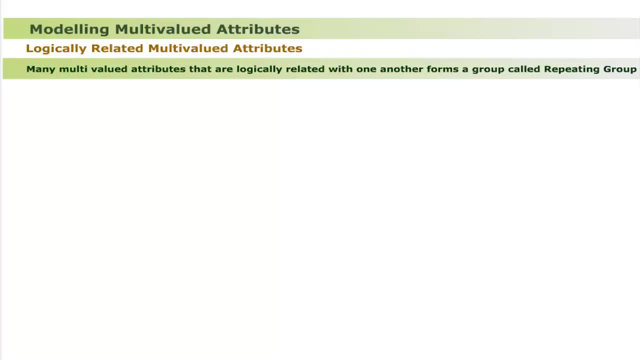 repeating group. These procedural steps are adopted to model a repeating group Number one. the repeating group is converted into new entity class Number two. the multi-valued attributes of original entity class become the attribute of newly created entity class Number three. the newly created entity class must have the composite key with primary key. 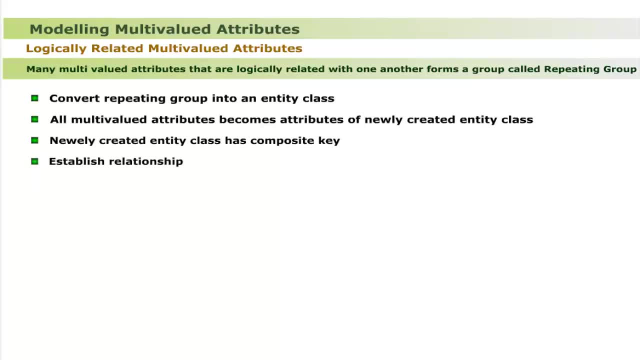 attribute of original entity class. Number four establish relationship between original entity class and newly created entity class. Let us examine entity class faculty. as shown, It has two single valued attributes- faculty code and name- and two multi-valued attributes- project code and registration number. 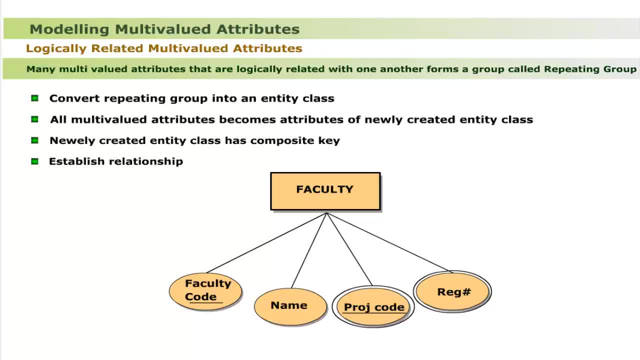 This model shows a faculty member supervises a number of software projects taken by students. Let us now examine how entity class faculty is modeled. Let us now examine how entity class faculty is modeled. the steps involved are the two multi-valued attributes, project code and. 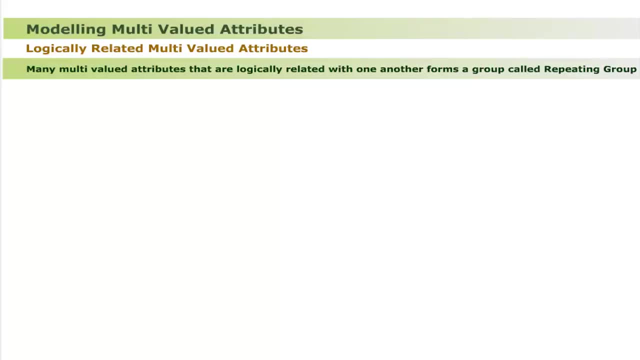 registration number are logically related, thus form a repeating group. this repeating group is converted into new entity class, project number two. the multi-valued attributes of original entity class, that are, project code and registration number, become attributes of newly created entity class, project number three. the newly created entity class, that is, project, have composite key. 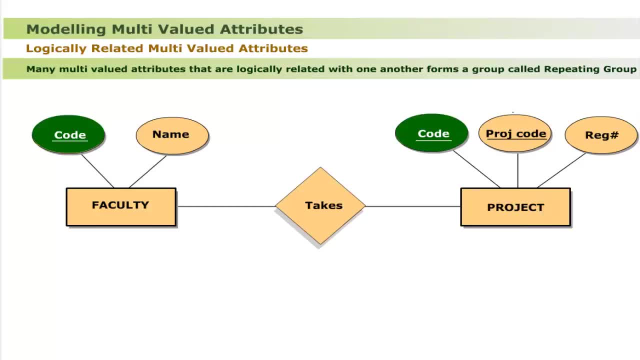 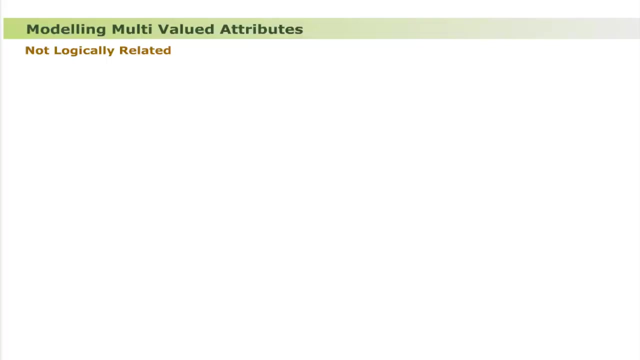 composed of attributes, project code and faculty code. the attribute faculty code is the primary key attribute of original entity class, that is, faculty number four. the relationship takes is established between original entity class, that is, faculty, and newly created entity class- project, not logically related. dear learners, let us now discuss the second possibility for existence of many 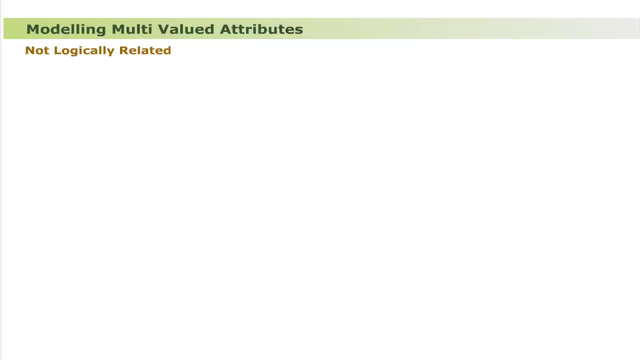 multi-valued attributes in an entity class. here is the detail: if there are many multi-valued attributes in an entity class not logically related, then these procedural steps are adopted to. model number one can work each multi-valued attribute into a new entity class. number two: the newly 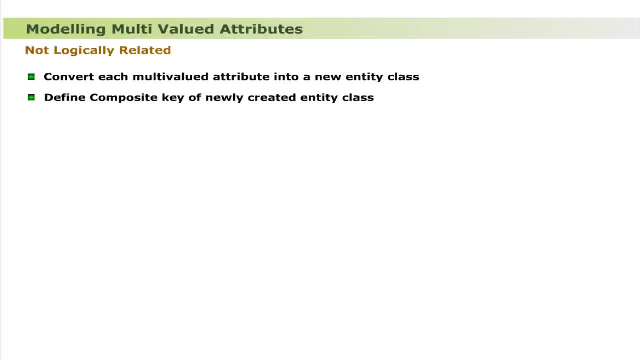 created entity classes must have composite key with primary key attribute of original entity class. number three established relationship between newly created entity class Entity Classes and the original Entity Class. Let us examine Entity Class Student as shown. It has two single-valued attributes- registration number and name- and two multi-valued attributes. 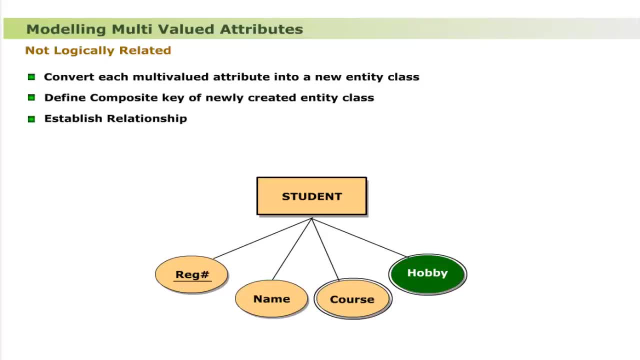 course and hobby. This model shows a student may register many courses and also have many hobbies. It is important to note that the course registration has no bearing on hobbies. Let us now examine how Entity Class Student is modeled. The steps involved are number. 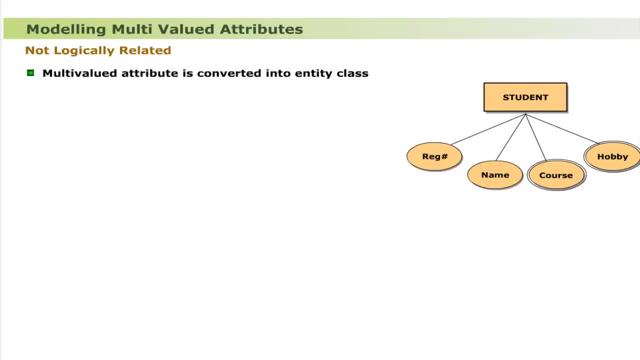 one: the multi-valued attribute course is converted into new Entity Class course. Similarly, multi-valued attribute hobby is converted into new Entity Class hobby. Number two: the newly created Entity Class course has composite key composed of attributes, course code and registration number. Similarly, the newly created Entity Class 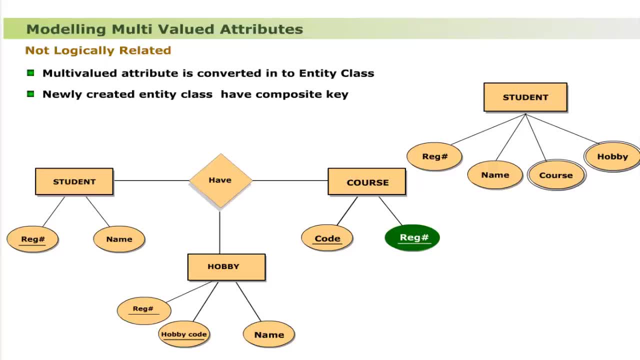 hobby has composite key composed of attributes: course code and hobby code. The attribute registration number in both the Entity Classes is a primary key of original Entity Class, that is student. Number three: the relationship have is established between original Entity Class that is student and two newly created Entity Classes that are course and hobby. 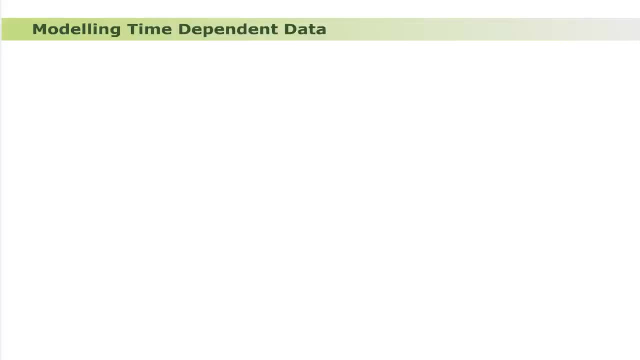 Modeling time-dependent data. Updating of data with the passage of time is frequently required in information science. Modeling time-dependent data is frequently required in information science. Modeling time-dependent data is frequently required in information systems. Sometimes previous versions of data values are required for future reference. 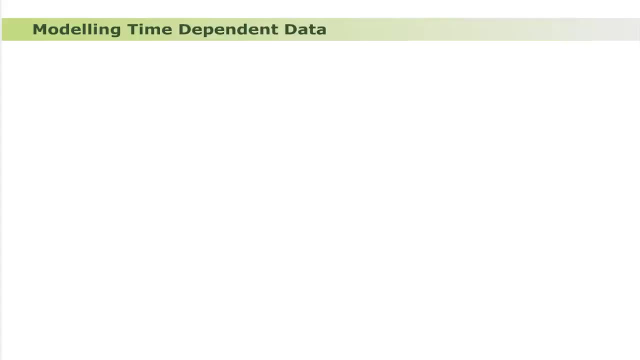 Such type of data, whose values are updated with the passage of time and the history of change values is kept, is called time-dependent data. For example, the fee per credit hour in a semester for BS program is Rs.1200, effective from Spring 2002 semester. The total fee is: 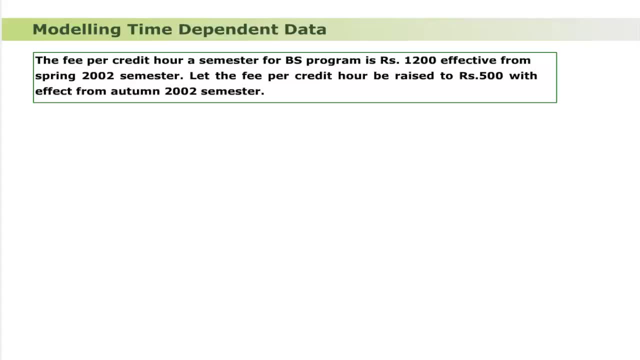 calculated by multiplying number of credit hours per semester by the number of credits and credit hours registered, with Rs.1200.. Let the fee per credit hour is raised by Rs.500 with effect from Autumn 2002 semester. The fee of a student in a subsequent semester. 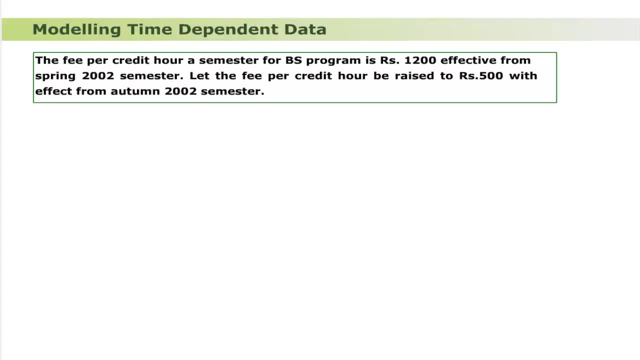 is calculated at the rate of per credit hour effective at the time of admission. In this case, the fee rate is revised with the passage of time and the history of changes is required to keep This data item is time-dependent. The time-dependent data always makes a repeating. 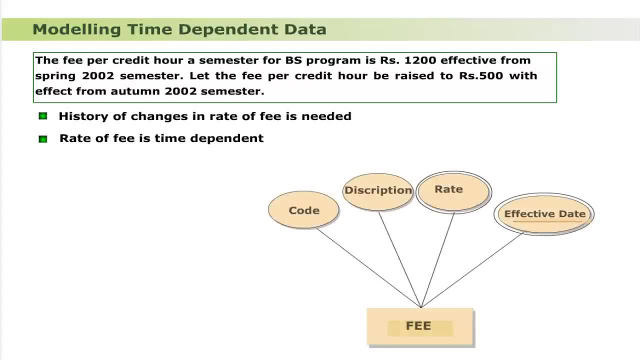 group. the entity class fee is shown as it has two single valued attributes- fee code and description- and two multi-valued attributes- rate and effective date. let us now examine how entity class fee is modeled. the steps involved are, number one, the two multi-valued attributes- rate and. 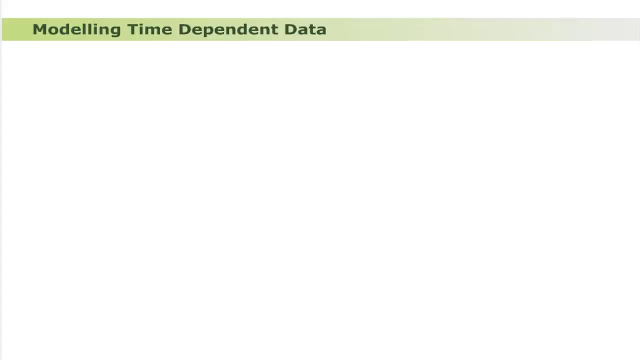 effective date are logically related, thus form a repeating group. this repeating group is converted into new entity class- history number two. the multi-valued attributes of original entity class that are rate and effective date, become attributes of newly created entity class, that is, history. number three: the newly created entity class, that is history, has composite key composed of: 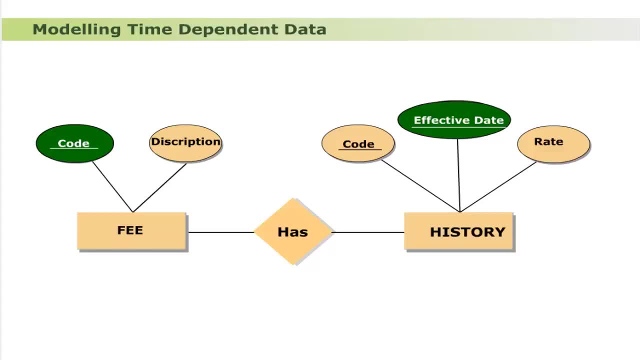 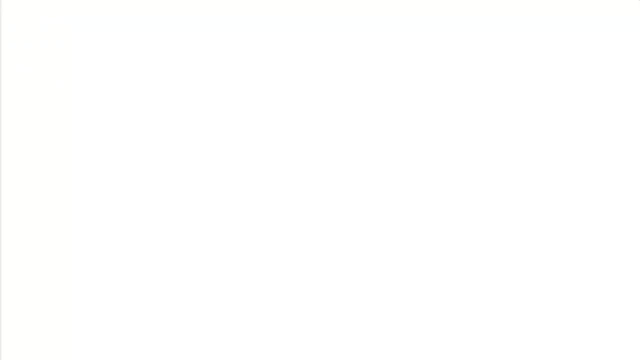 attributes: fee code and effective date. the attribute fee code is the primary key attribute of original entity class, that is, fee, number four. the relationship has established between original entity class, that is, fee, and newly created entity class history Gerand. the relationship of type many to many between entity classes when converted into an entity class is called gerand. it. 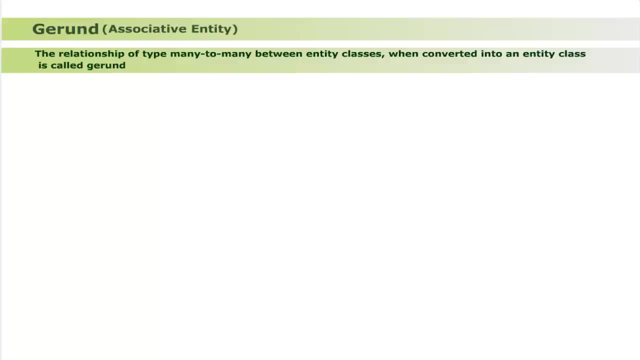 is also called associative entity. the reason of converting such a relationship into an entity class is discussed in the subsequent example. here is the example. many students register many courses in a given semester. The formation of gerund is given stepwise as Step 1. The single entity class student is shown as: 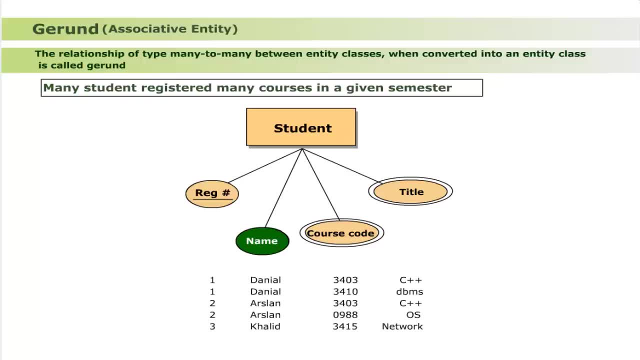 It has two single-valued attributes- registration number and name- and two multi-valued attributes- course code and title. There is high degree of redundancy due to existence of multi-valued attributes: course code and title. These multi-valued attributes need a refinement as in Step 2.. 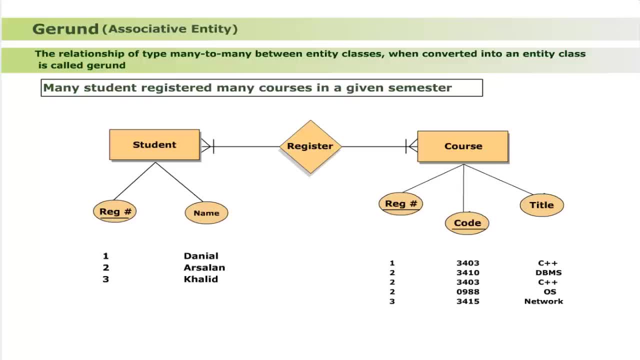 The multi-valued attributes are converted into the associative entity course with attributes registration number, course code and title, as shown. Let us examine this refined modelling. The redundancy pointed out in Step 1, is reduced as the name of student is stored once, even registered, in many courses. 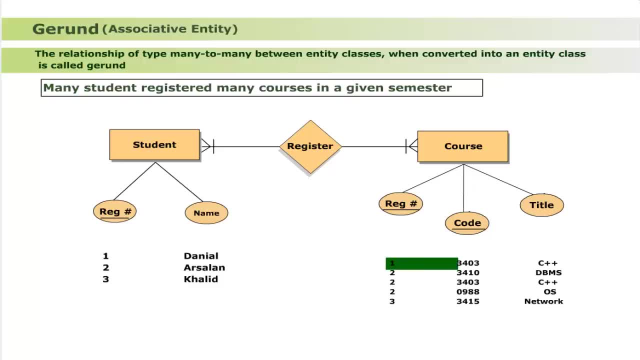 But the entity course has still a redundancy, ie the title C+, Correct- is duplicated. Dear learners, it is a point to think why there is redundancy. The reason for this redundancy is the existence of relationship register of type many-to-many between entity. 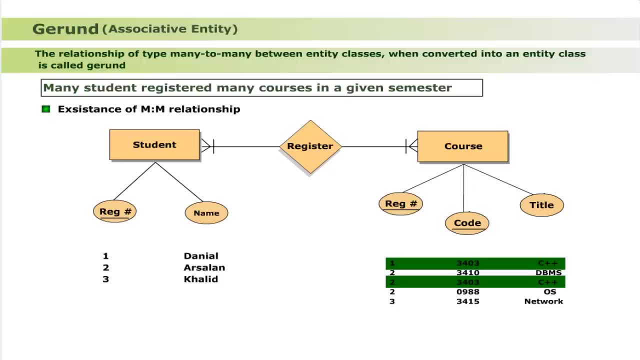 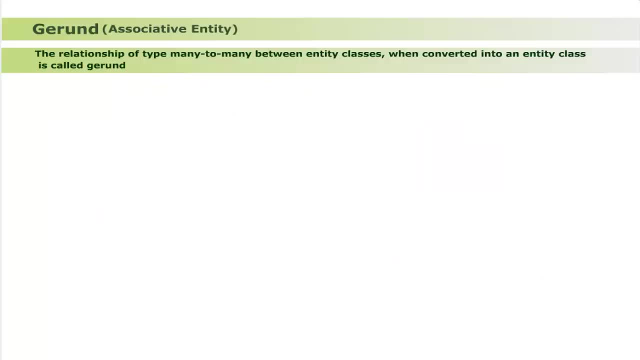 classes, student and course. Now it is time to learn how such problems are solved. Here is the detail: Whenever there is a relationship of type many-to-many, it is converted into new entity class called associative entity, also called gerund, such that there must be a composite key. 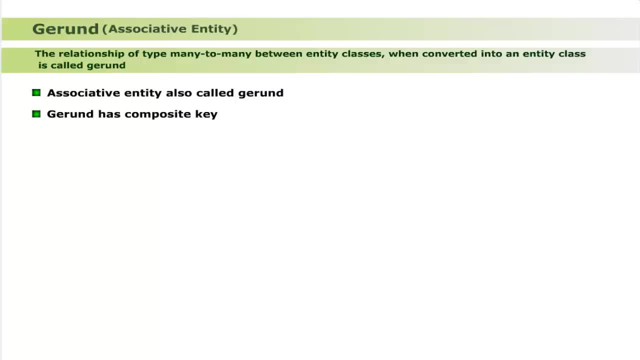 which must be constructed by the primary keys of all associated entity classes. It may also have non-key attributes. The general representation of associative entity is shown as Dear learners. the model as shown is refined further in order to control redundancy. as shown The relationship. 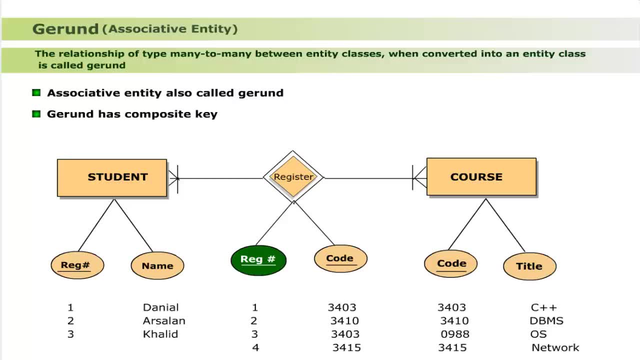 register is converted into new entity class called associative entity, also called gerund. The model is then converted into associative entity with attributes registration number and course code, which collectively forms a composite key. Now let us evaluate the model for any redundancy as existed before. The name of any student is stored once, no matter how many. 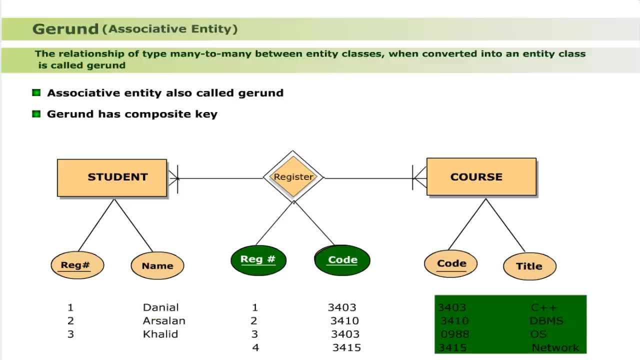 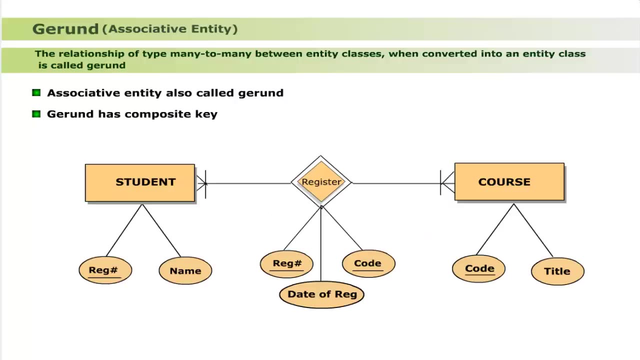 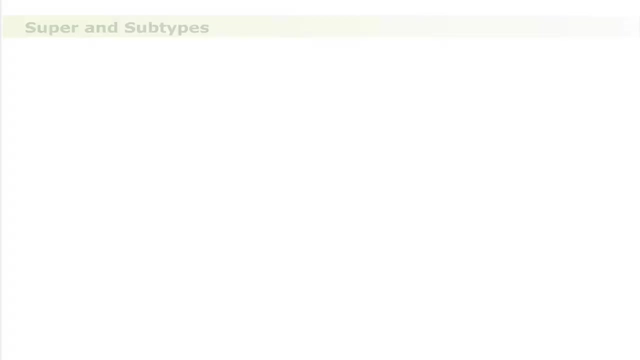 courses does he register? Similarly, the course title is stored once, no matter how many students register that course. Thus the gerund, or associative entity, greatly controls redundancy. Dear learners, the gerund may also have non-key attributes, as shown Super and subtypes. Dear learners, let us first discuss the concept of super and subtype. In most, 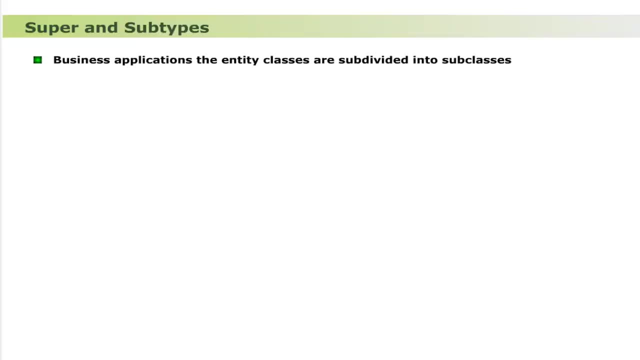 business applications. the entity classes are subdivided into subclasses. This subdivision is generally done for easy administration and management. For example, a university is considered as an entity class university. This entity class as a whole is very complex and difficult to administer. Therefore it is further subdivided into subclasses that 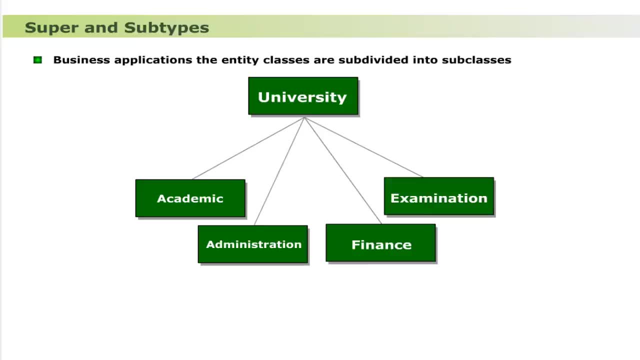 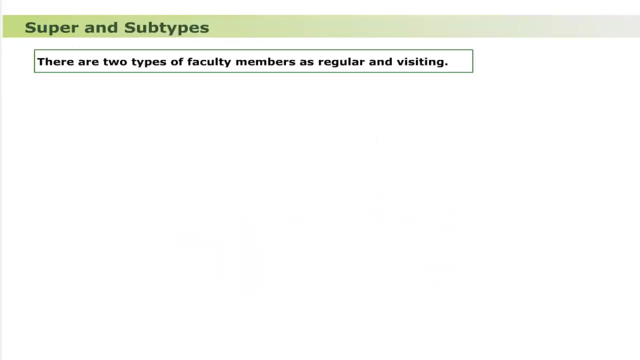 are academic administration, finance, examination and many more. The generic entity class, which is further subdivided into subclasses, is called supertype and each subclass of a superclass is called subtype. The ER representation of super and subtype is shown as: Let us consider this example. There are two types of faculty members, as regular and visiting. 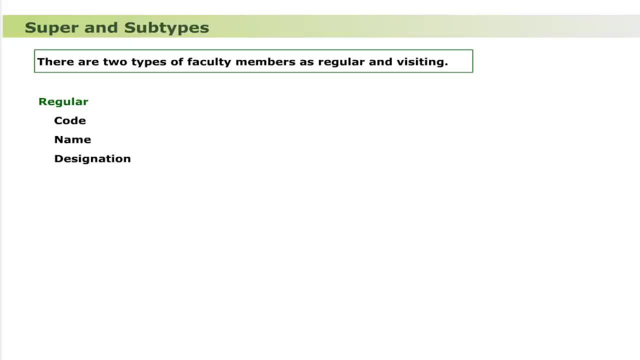 The attributes of regular faculty member are employee code, employee name, designation and salary per month. The attributes of visiting faculty members are employee code name, teaching rate per hour and contract period. Dear learners, now it is time to examine how the given situation 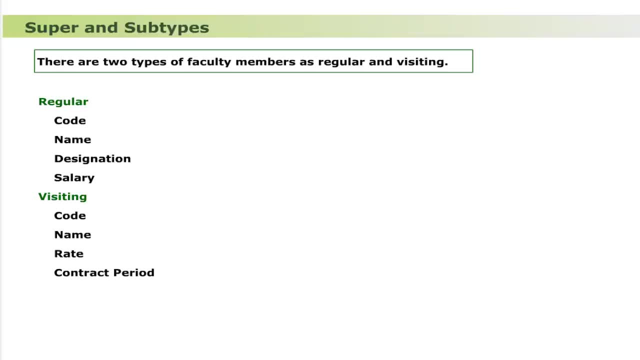 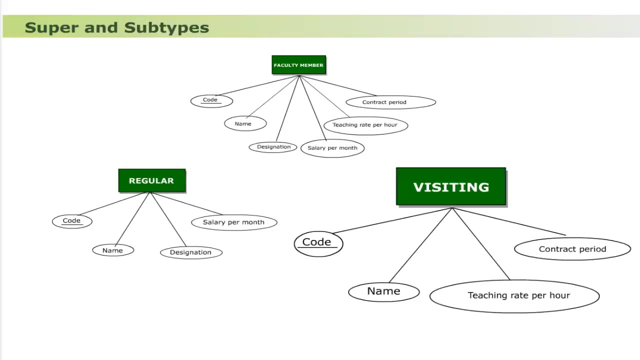 is modeled. Let us model it on the basis of what we learned previously. There are two choices for depicting the ER model. Number one: define one entity class faculty member as shown. Number two: define entity class regular for regular faculty and visiting for visiting. 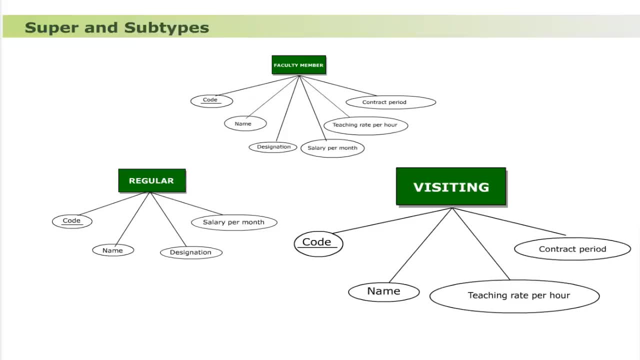 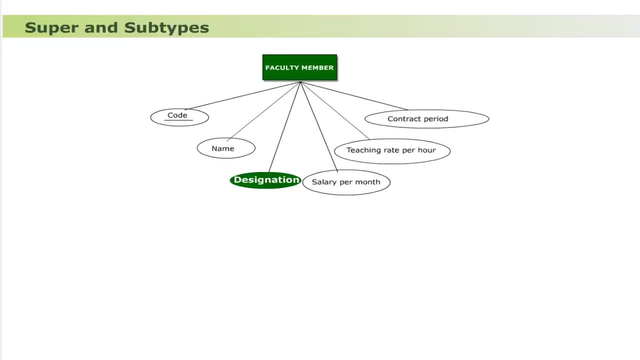 faculty as shown. Let us examine both the models. The single entity class faculty member has a drawback that there are some attributes which are not applicable to every faculty member. For example, the attribute designation is not applicable to an instance of faculty member. The attribute designation is not applicable to an instance of faculty member of the type: 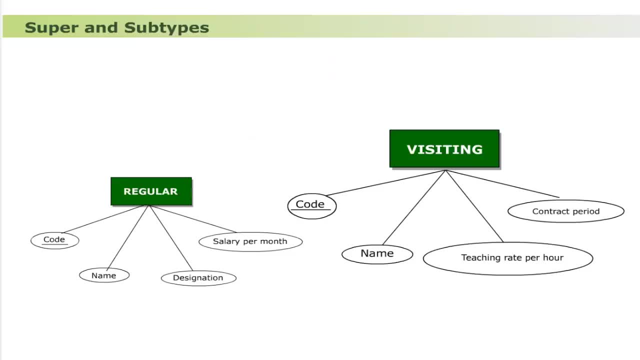 visiting, as shown, The two entity classes that are regular and visiting, has a drawback that common attributes, that are employee code and name, are defined with each entity class. Thus the commonly existed attributes are defined redundantly, Dear learners. now what must be done to resolve the stated problem with each model? 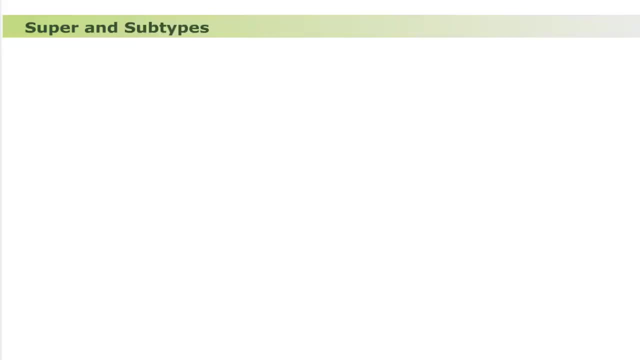 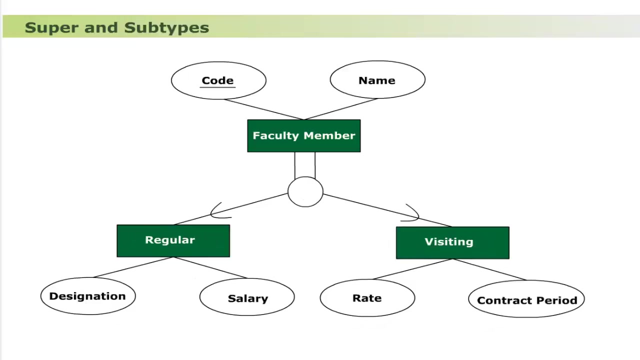 The concept of super and subtype discussed is the key to refine the stated models. The super and subtypes are modeled as: define supertype with attributes common to all defined subtypes. Define subtypes with attributes unique to each subtype. Now let us use the concept of super and subtype in the stated model. 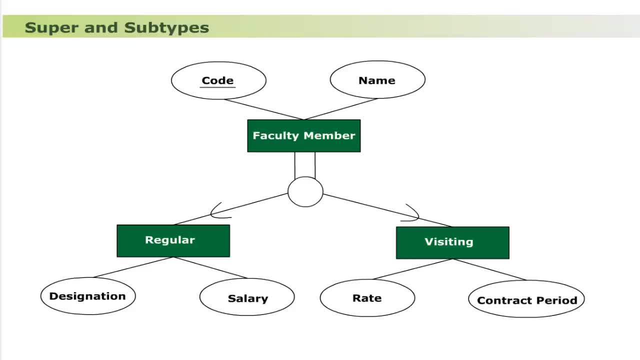 Define supertype faculty member and subtypes regular and visiting. The attributes of supertype faculty member are employee code as primary key and name. The attributes of subtype regular are designation and salary. Similarly, the attributes of subtype visiting are as primary rate per hour and contract. 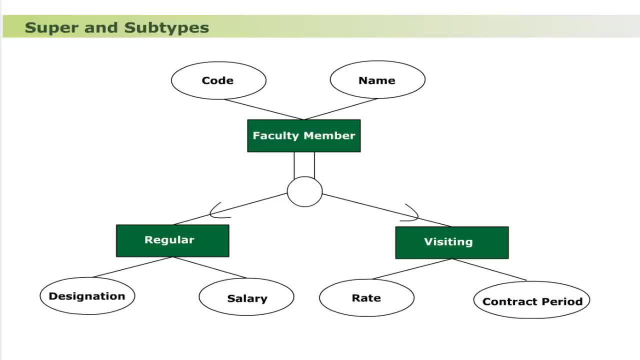 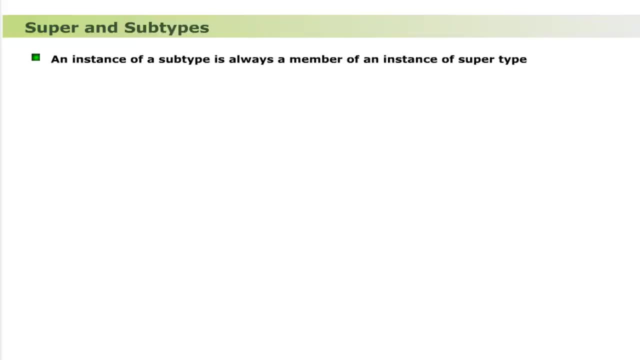 period. Dear learners, dealing with super and subtypes, it must be kept in mind that an instance of subtype is always a member of an instance of supertype. The subtype inherits values of all attributes of supertype. So far we learned that a generic entity is modeled as super and subtypes. if all subtypes 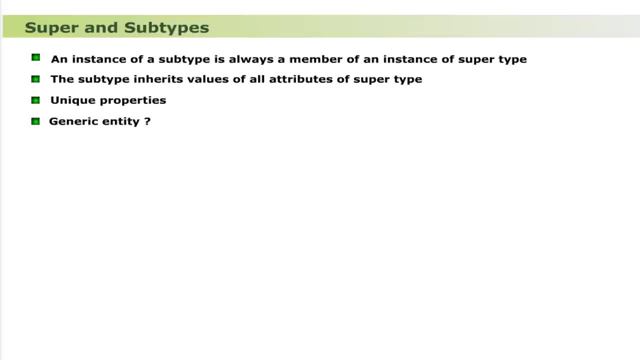 have unique properties. But what about a generic entity if subtypes have same attributes, Dear learners? such type of a generic entity is modeled as single entity class with an additional attribute for differentiating the type. For example, consider the situation. There are two types of students studying in morning shift or evening shift. 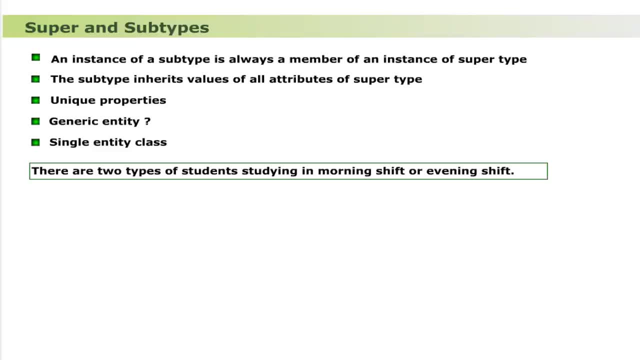 The attributes of student are registration number, name and city. The student entity class must not be modeled as super and subtype, but rather be modeled as single entity class, as shown. The attribute shift is an additional attribute defined to differentiate the type of student: either morning or evening. 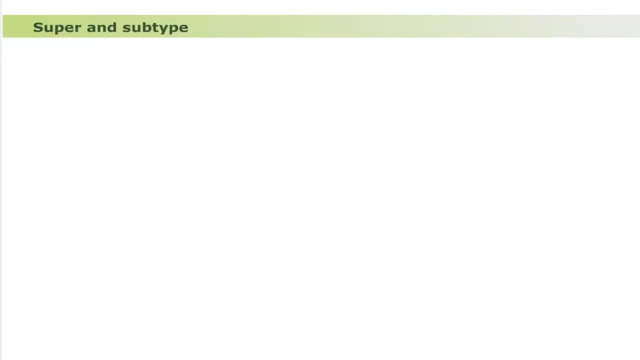 Specialization and Generalization. Dear learners, so far we discussed the basic principles of super and subtypes modeling, But in developing real-world data models, how can we recognize the opportunities to explore the super and subtype relationship? There are two processes, Two processes which serve as mental model in developing super and subtypes relationships. 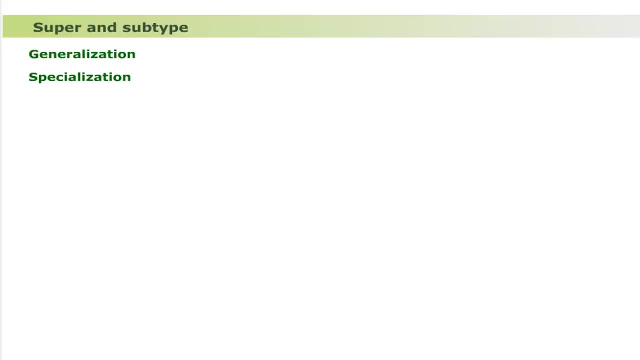 These are: generalization, specialization. Let us discuss each one in detail. Generalization In data modeling: the generalization is the process of defining a more general entity from a set of more specialized entity types. For example, consider these three entity types as shown. 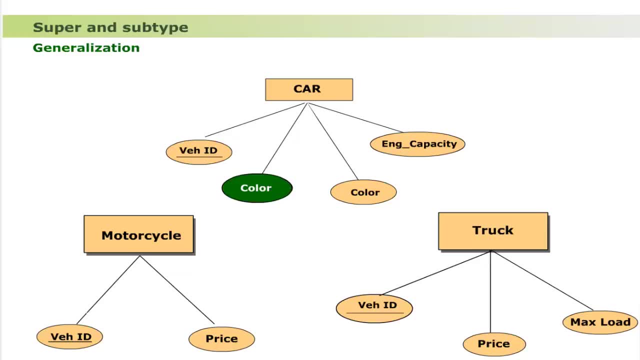 The entity car has attributes Vehicle identification number, Color, Price And engine capacity. The entity motorcycle has attributes Vehicle identification number and price. The entity truck has attributes Vehicle identification number, price and maximum load. It becomes clear by closely examining these entities that the attributes vehicle identification 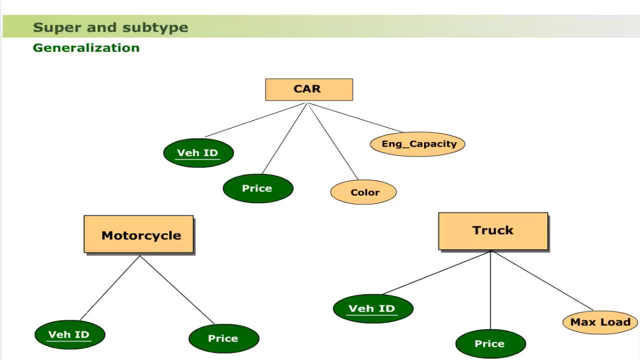 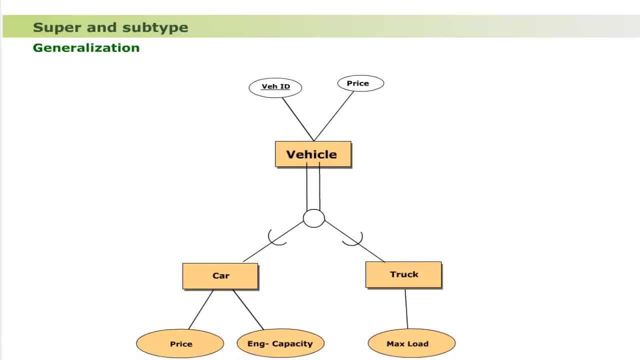 number and price are common. This fact reiterates that each of the given entity types is a version of more general entity type vehicle. as shown, The entity car has attributes, Color, Price And engine capacity. It inherits all attributes of its supertype vehicle as it is an instance of it. 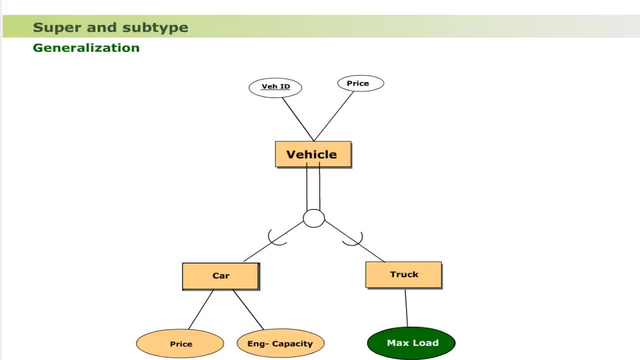 Similarly, the subtype truck has attribute maximum load. It also inherits all attributes of its supertype vehicle as it is an instance of it. Dear learners, the entity type motorcycle is missing here. Is this simply an omission? No, It is deliberately not included. 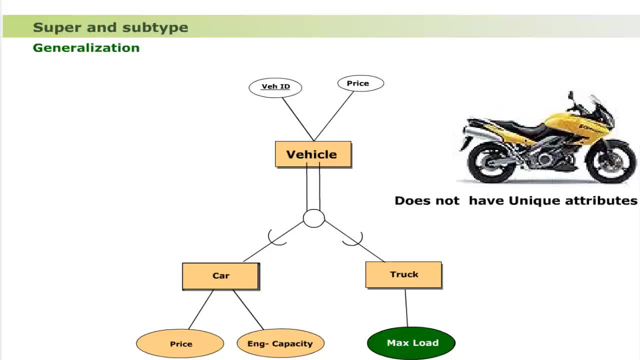 Because it does not satisfy the condition for us. The entity type motorcycle is missing here. Thus it is now an exception Here also we find that the entity type motorcycle does not have a unique attribute, It is just a subject. The specific attribute of a vehicle type motorcycle is a subtype. 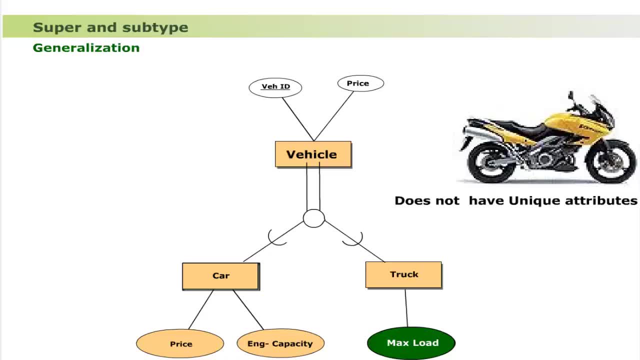 The motorcycle entity type does not have unique attribute. It has to be presented for existence as subtype of a supertype. It has to be presented for existence as a subtype of a supertype. The absence of motorcycle entity type also shows that an instance of a supertype is not necessarily 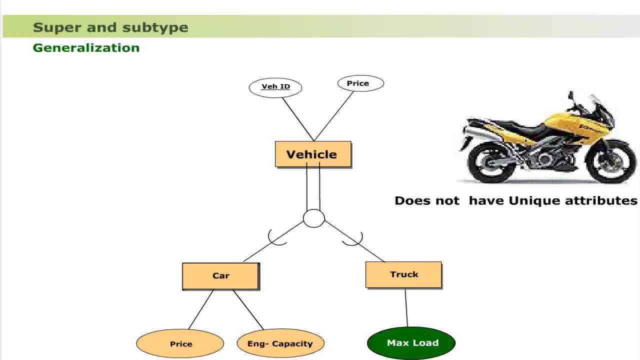 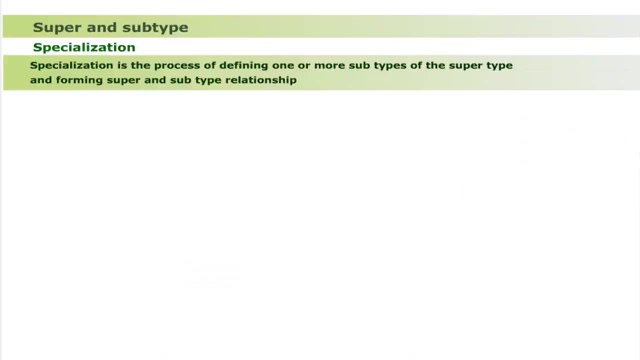 a member of any of the defined subtypes. This is discussed further in the next section. Now is the time to discuss the second process of mental model in developing super and subtypes relationships, eg Specialization. In data modeling, the specialization is the process of defining one or more subtypes of the supertype and forming super and subtype relationship. 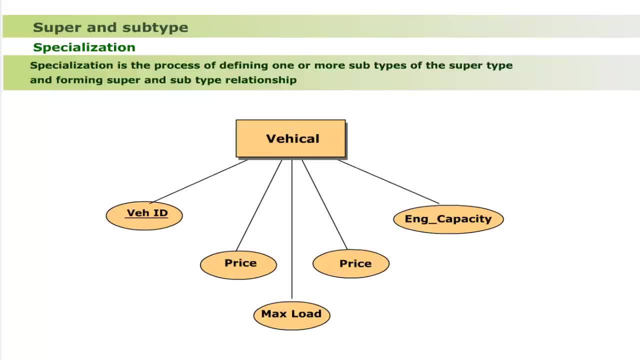 For example, consider the entity type vehicle. The attributes are vehicle identification number as primary key, price, color, engine capacity and maximum load. After further discussion with user of these vehicles, it is discovered that two types of vehicles are used. Each has unique attributes. 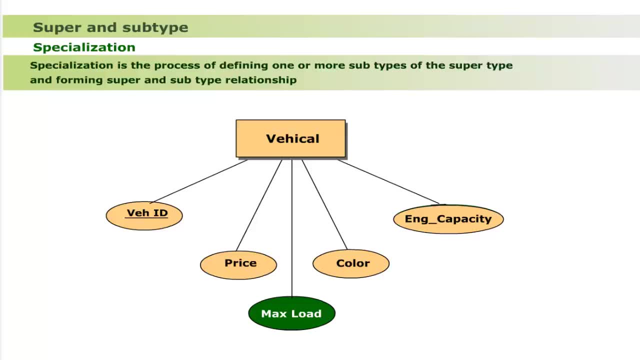 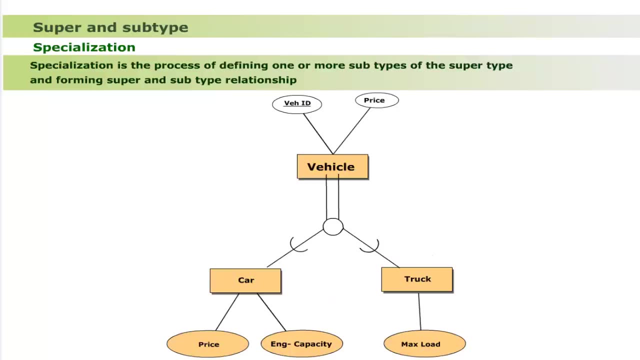 The domain of stated problem clearly demonstrates that the most general entity type vehicles shall be decomposed into more specialized subtypes, each with unique attributes, as shown. Dear learners, now it is clear that generalization and specialization are two techniques used for modeling of super and subtypes. 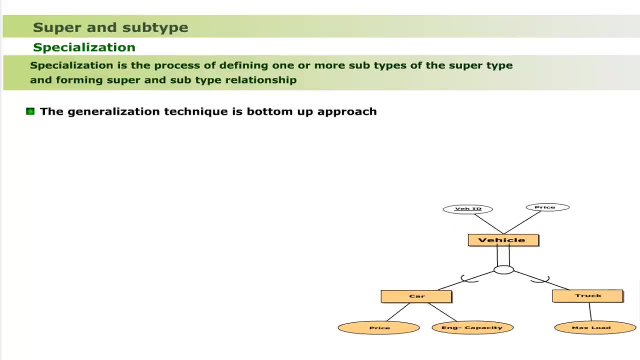 These are the two main techniques used for modeling of super and subtypes. These are the two main techniques used for modeling of super and subtypes. These are summarized as: the generalization technique is bottom-up approach, while the specialization technique is top-down approach. 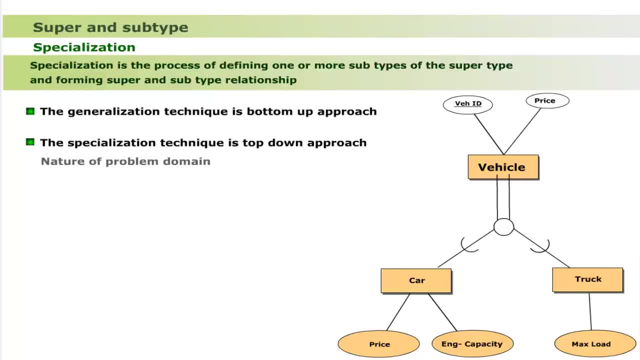 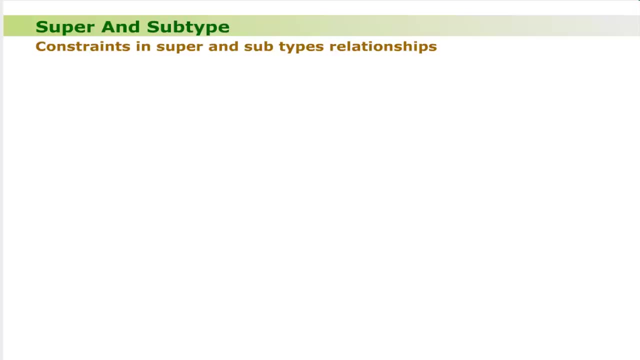 The application of either of these techniques depends upon nature of problem domain, previous modeling efforts, if any, and maybe personal preferences, Constraints in super and subtypes relationships, Dear learners, so far we discussed the basic principles of super and subtypes modeling and concept of 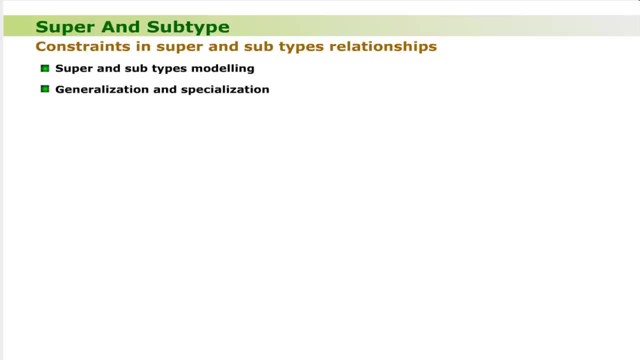 generalization and specialization. But very often there are constraints which help to apply important business constraints to super and subtype relationships. These are completeness constraint and disjointness constraint. Let us discuss each in detail. The completeness constraint addresses the question whether an instance of a supertype must also be a member of at least one subtype. 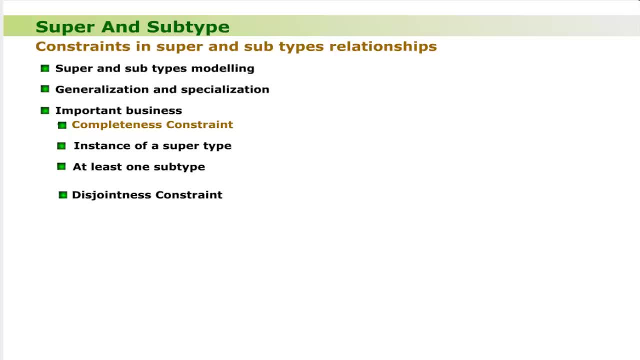 The completeness constraint has two specialization rules. These are total specialization and partial specialization. Let us discuss each one in more detail. The total specialization rule specifies that each instance of supertype must be a member of some subtypes of the supertype. The general representation is shown as: 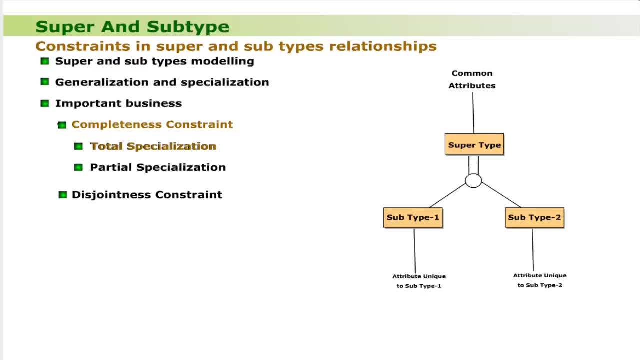 the two parallel lines that join supertype entity to small circle shows that total specialization. For example, consider there are two types of employees that are regular and contract. Each type has some common attributes and unique attributes. The common attributes are employee code as identifier, name and designation. 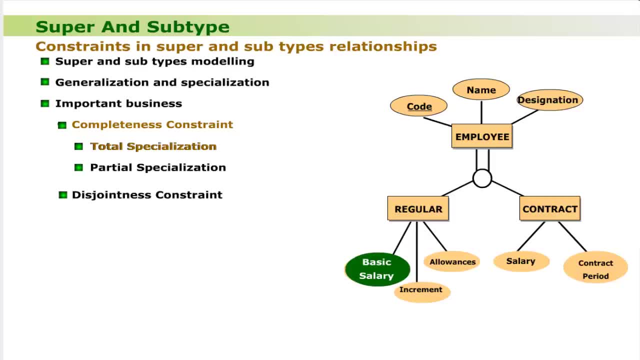 The unique attributes of regular employee are basic salary, annual increment and allowances total. The unique attributes of contract employee are total salary and contract period. Dear learners, in order to model this example, we first analyze it On the basis of our previous learning, as the problem domain shows that super and subtype relationship must be applied to model it, and either of specialization or generalization technique could be used. 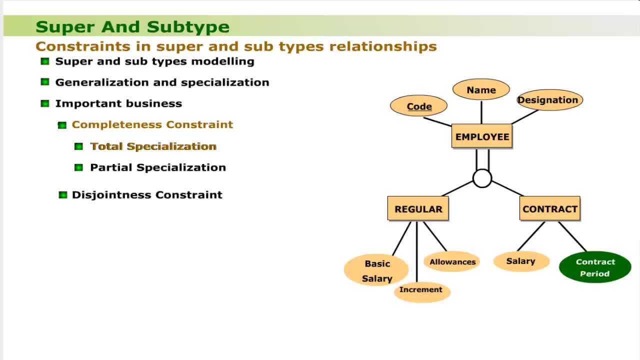 The problem domain also shows that an employee that is an occurrence of supertype is necessarily the either of the two defined subtypes that are regular or contract, but never both at the same time and there is no other type. This shows that total specialization rule is applied. 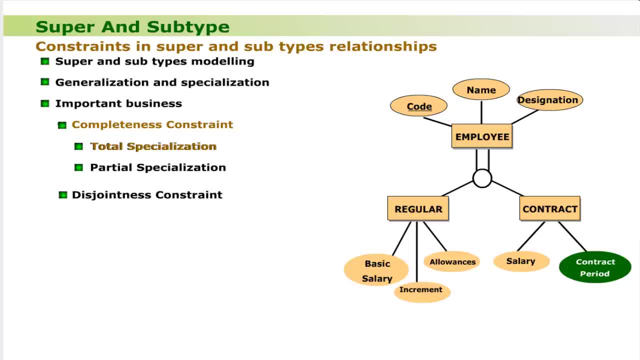 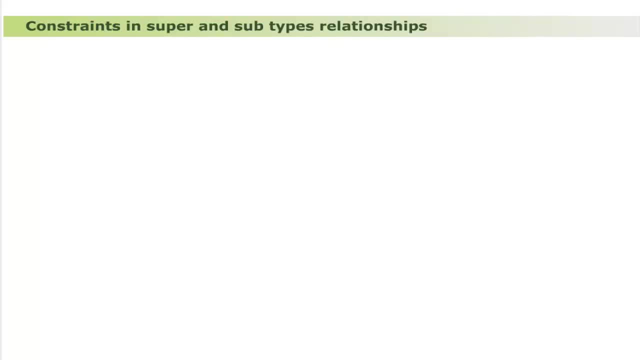 The super and subtype model of the stated problem is shown as Dear learners, let us now discuss the second rule of completeness constraint, that is, Partial specialization. The partial specialization rule specifies that an instance of supertype does not belong to any of the defined subtypes. 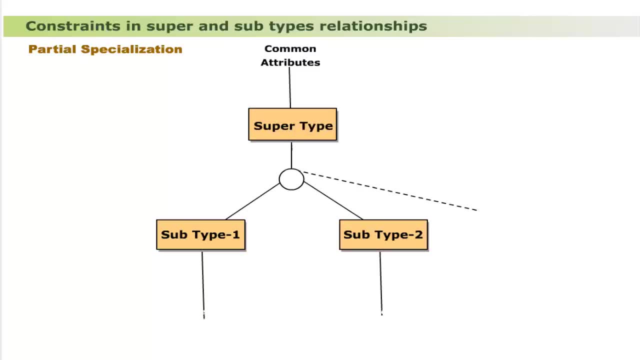 The general representation is shown as The single line that joins the supertype entity to a small circle shows the partial specialization. For instance, let us modify the employee example just discussed in total specialization as The organization generally has two types of employees: regular and contract. 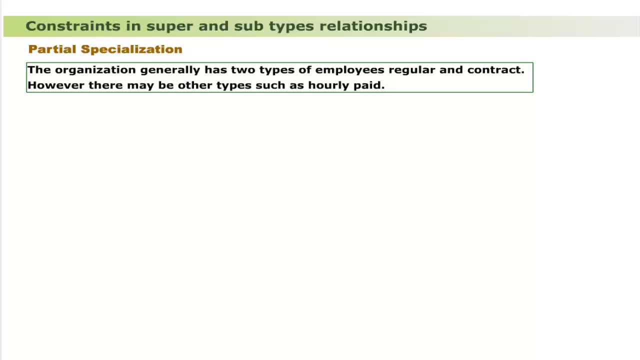 However, there may be other types also, such as hourly paid. Dear learners, in order to model, this time we first analyze it on the basis of our previous learning, as The problem domain shows that super and subtype relationship must be applied to model it. 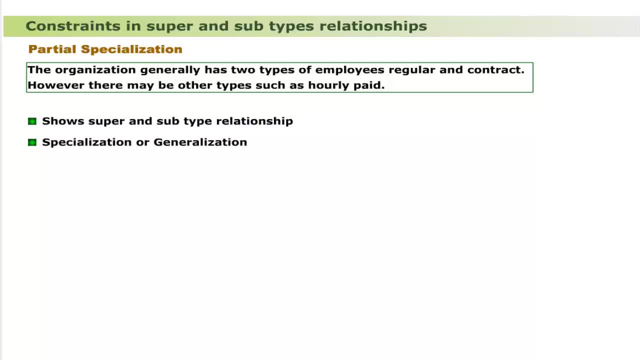 and either of specialization or generalization technique could be used, for example. or generalization technique could be used. the problem domain shows that an employee that is an occurrence of super type is not necessarily belong to either of the two defined subtypes that are regular or contract, but may also be of 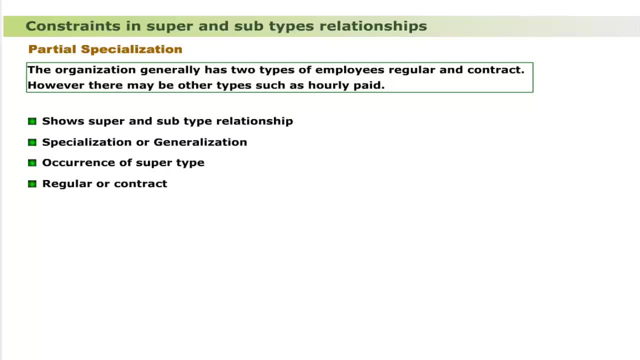 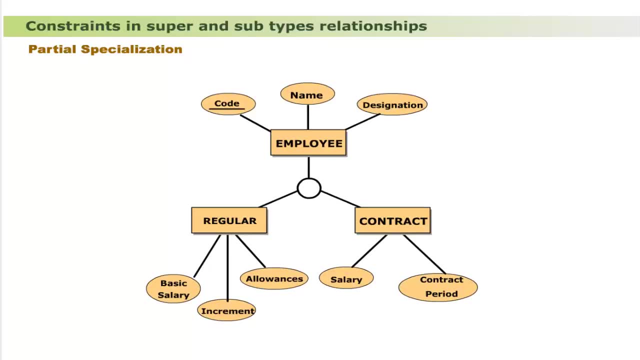 other undefined type. this shows that partial specialization rule is applied. the super and subtype model of the stated problem is shown as dear learners. after discussing the completeness constraint, now let us discuss the disjointness constraint. the disjointness constraint addresses the question whether an instance of super type simultaneously is a member of two. 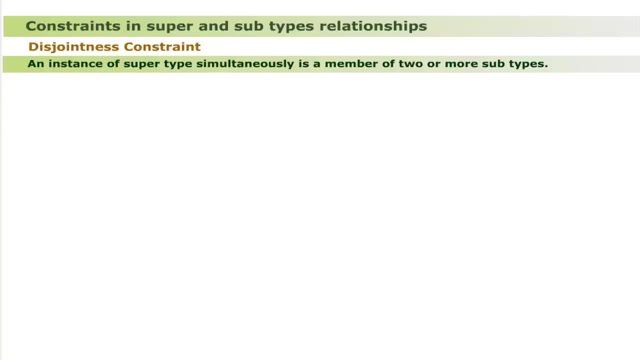 or more subtypes at the same time. it has two rules. these are disjoint rule and overlap rule. let us discuss each in more detail. the disjoint rule specifies that an instance of super type must match to only one of the subtypes either defined or undefined. it is represented in two. 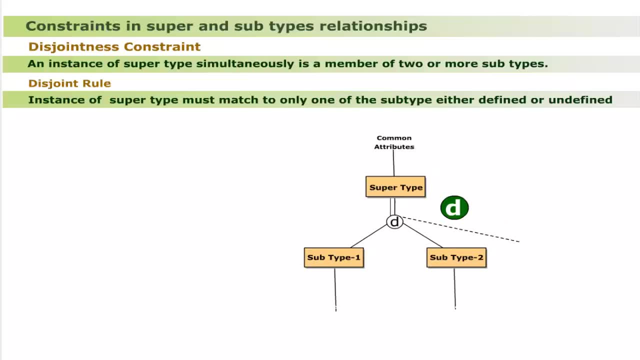 ways as shown. the small circle with D inside shows disjoint rule. the parallel lines show that there is no other subtype except the defined subtypes. for example, let us modify slightly the employee example discussed earlier in total specialization. here is the modified model. as shown, the employee is: 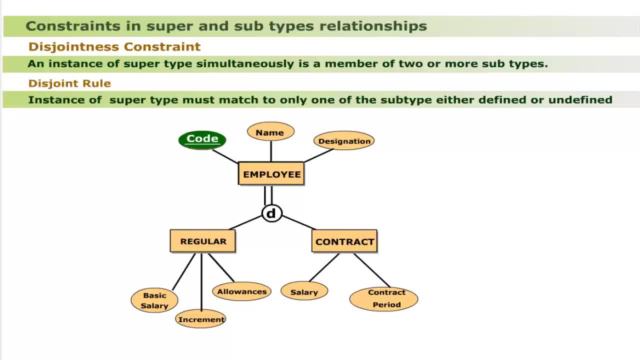 the super type: entity with common attributes: employee code as identifier, name and designation. there are two subtypes: regular, with unique attributes- basic salary, annual increment and allowances total. and contract, with unique attributes- total salary and contract period. the model shows that an instance of employee is necessarily matched with either of. 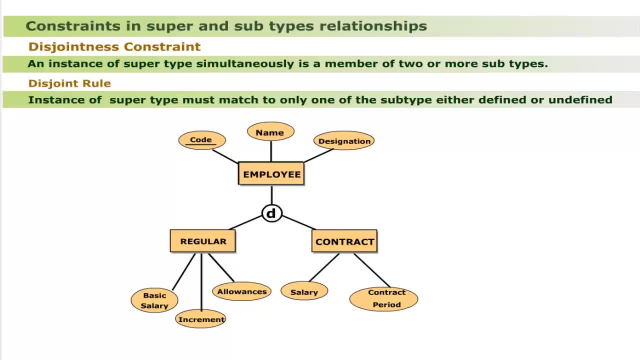 the two defined subtypes: regular or contract. dear learner, this is second representation. the small circle with D inside shows disjoint rule. the single line shows that there may also be subtypes other than the defined subtypes, for example disjoint rule. division D is defined mostly by disjoint rule deliberation. 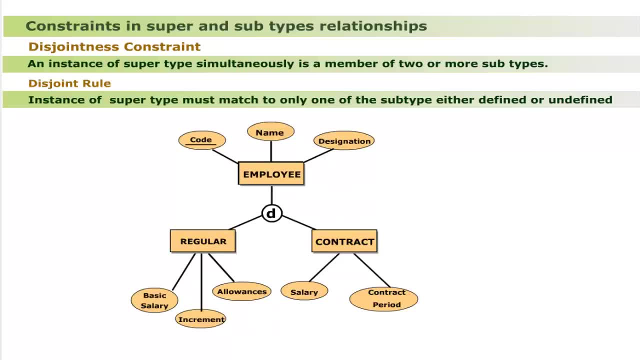 the SCG based method is defined in this simulation with elements 직 unit and unit D. in case any subtype change, it is выступ all data and int 얘. the sum of a subtype of are dogs. Yes, in this demonstration I shall discuss the wink from the 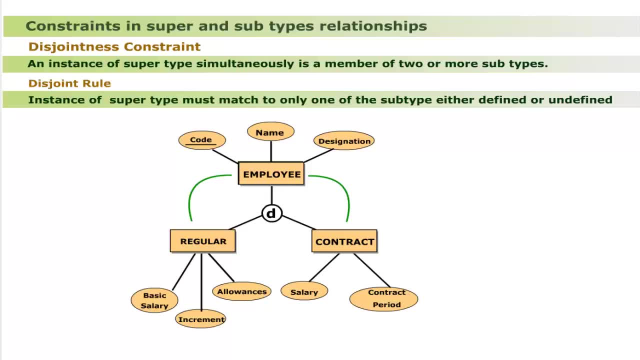 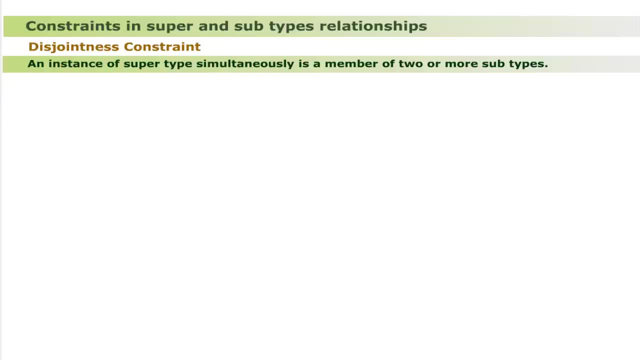 with either of the defined subtypes- regular and contract, or any other subtype not defined. Dear learners, after discussing the disjoint rule, now it is time to discuss the overlap rule. The overlap rule specifies that an instance of supertype may match to one or more of the subtypes. 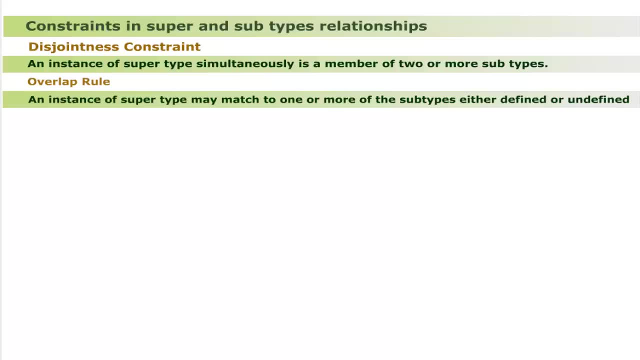 either defined or undefined. It is also represented in two ways, as shown. The small circle with O inside shows overlap rule. The parallel lines show that there is no other subtype except the defined subtypes. for example, Consider: there are three types of sport teams that are cricket, hockey and football in a sport club of a college. 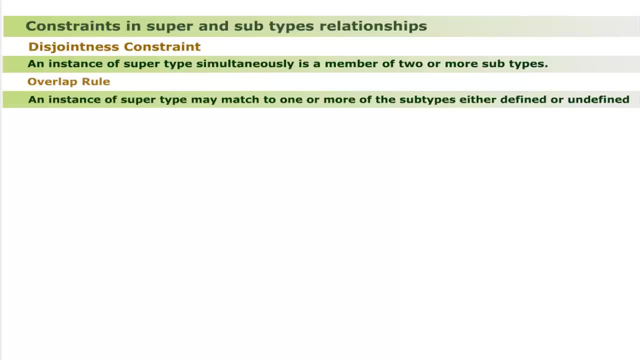 Each team has some unique attributes. Every member of the sport club is allowed to be member of more than one team. Here is the ER model. The model shows that an instance of sports club is necessarily matched with one or more of the defined subtypes: hockey, cricket or football. 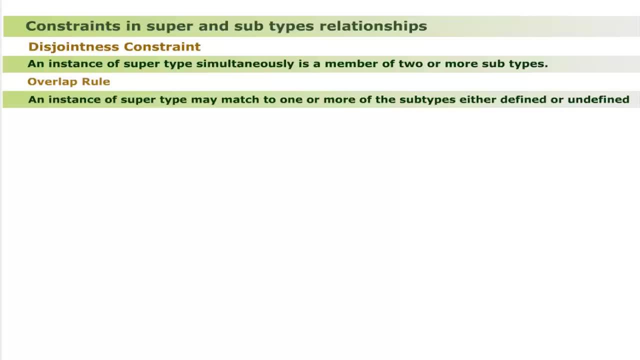 Dear learners. the second representation of overlap rule is shown as The small circle with O inside shows overlap rule. The single line shows that there may be other subtypes other than the defined subtypes. For example, let us modify the sports club example just discussed. 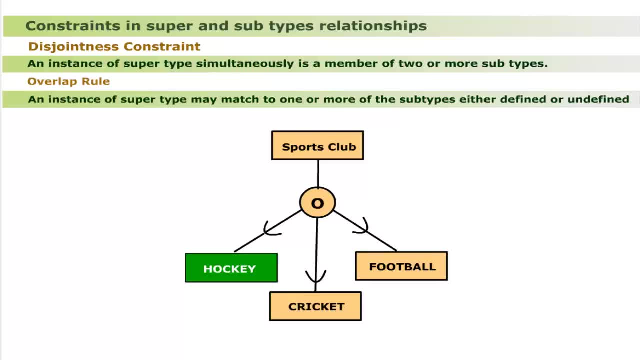 There are three types of sport teams. that are cricket, hockey and football. in a sports club of a college. Each team has some unique attributes. Every member of the sport club is allowed to be a member of more than one team and may be member of a team. 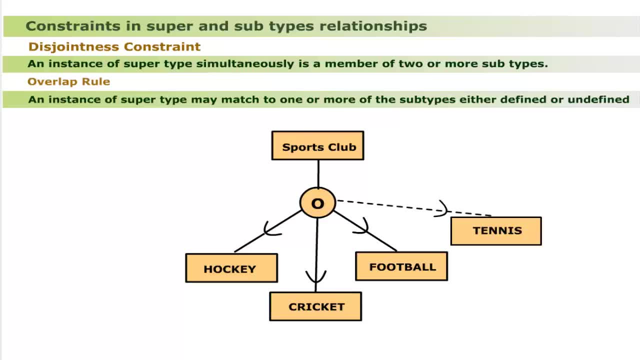 undefined as subtype, such as tennis. Here is the ER model. The model shows that an instance of sports club is necessarily matched with one or more of the defined subtypes- hockey, cricket and football- and other subtypes undefined, such as tennis. Hierarchical data model. The hierarchical data model is used to define the subtypes of sports clubs. Hierarchical data model was the first data model used for database design and implementation. In this data model, the entity classes are organized as a set of nodes in hierarchical manner. 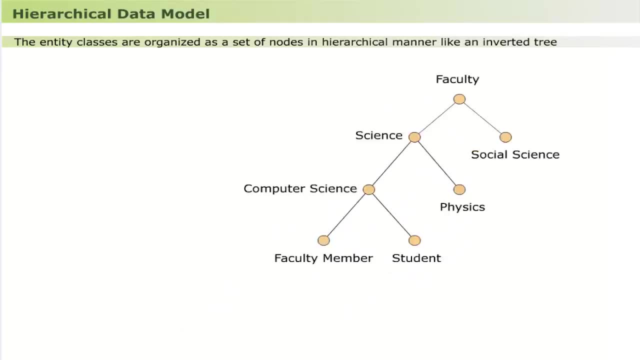 like an inverted tree structure as shown Here are few features of hierarchical data model. The entity classes are represented as a set of nodes. The entity classes are arranged in inverted tree-like structure starting from top node called root node. The nodes are linked physically through pointers. 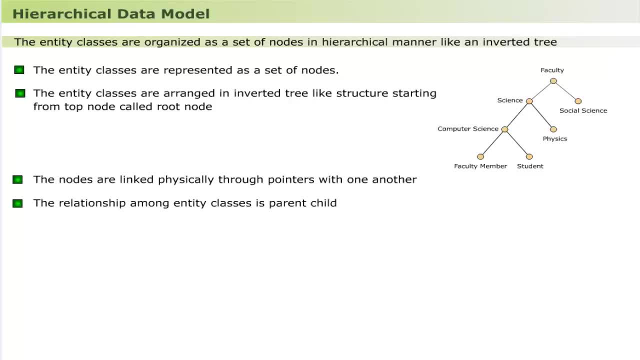 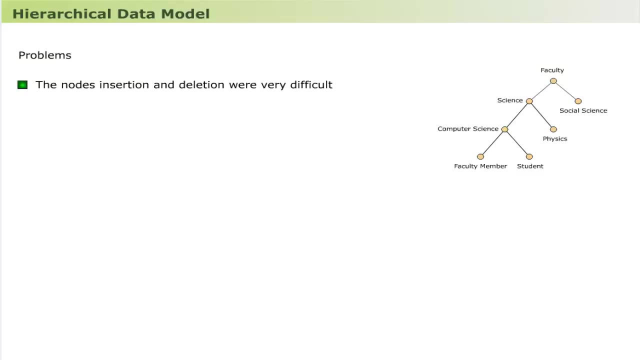 and the pointers with one another. The relationship among entity classes is parent-child, Dear learners. although hierarchical data model was very popular in the early era of database, however, the designer faced certain problems such as the nodes. insertion and deletion was very difficult. 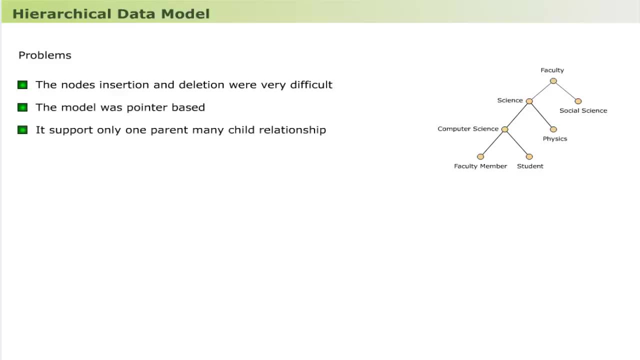 the model was pointer based. it supported only one parent-mini-child relationship. the model was rigid and static in nature. there was high degree of redundancy, But with the passage of time and advancement in the field, these problems were slightly overcome with the introduction of network data model. 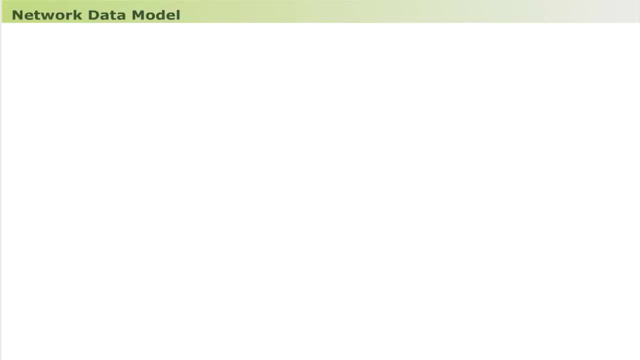 Network data model. In the network data model the entity classes are organized as a set of nodes, where any node could be connected or linked with any other nodes. as shown, The network data model preferred over hierarchical data model because of less redundancy and elimination of one parent-mini-child relationship. 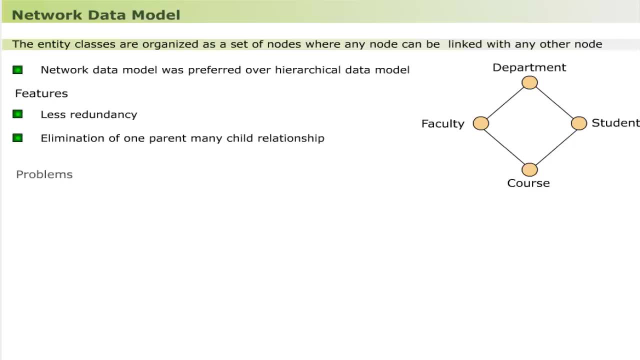 However, the designer was still faced with certain problems, such as the nodes. insertion and deletion was very difficult. the model was still pointer based. the model was still rigid and static in nature. These problems were overcome with the introduction of relational data model. Relational data model. 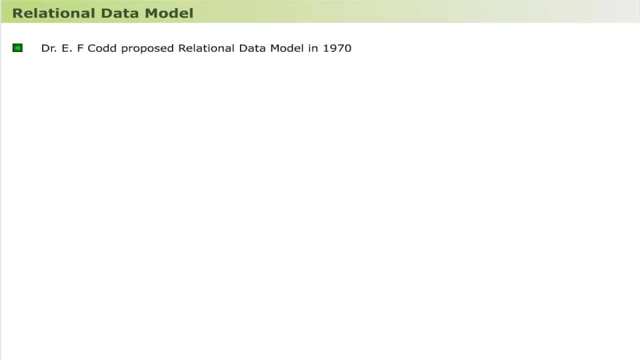 Dr E F Codd first introduced the relational data model in 1970, and it is still in use. In this model, the entity classes are represented as a set of relations or tables, as shown. The representation of table starts with the name of table. 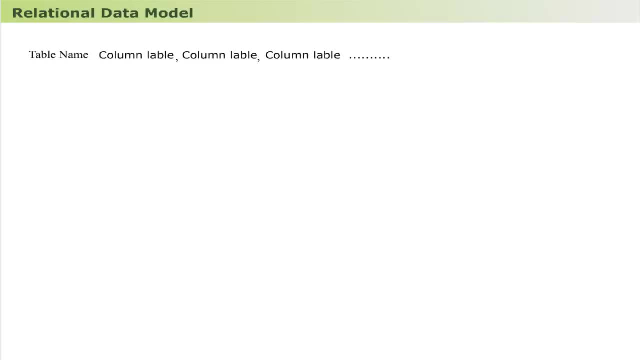 followed by column labels separated by comma and closed in parenthesis. For example, the table named student having three columns labeled: registration number, name and city as shown. The sample instances are shown as Relation. Dear Learners, Let us discuss the term relation, also called table, in more detail. 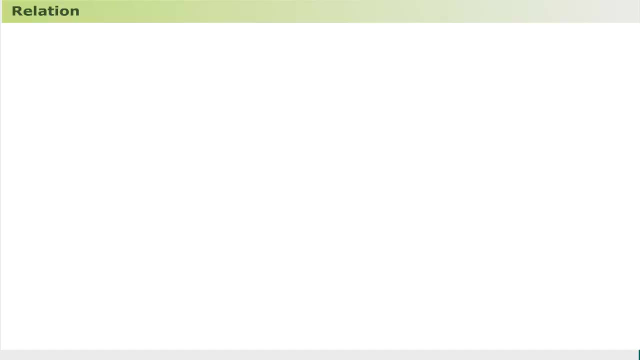 The relation is the basic building block of relation data model. The term relation is defined as It is a named two-dimensional set of data represented as unnamed rows and named columns. Every relation, whether simple or complex, has certain properties. These are: Every relation has a unique name. 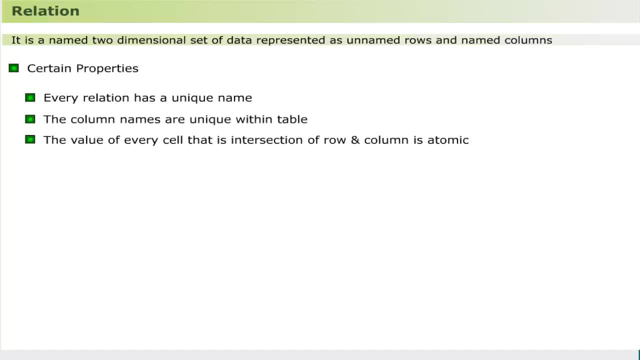 The column names are unique within table. The value of each cell, that is, intersection of a row and column, is atomic. There must be primary key or composite key, but never both at the same time. This ensures that every row is unique. The rows may be viewed in any required order. 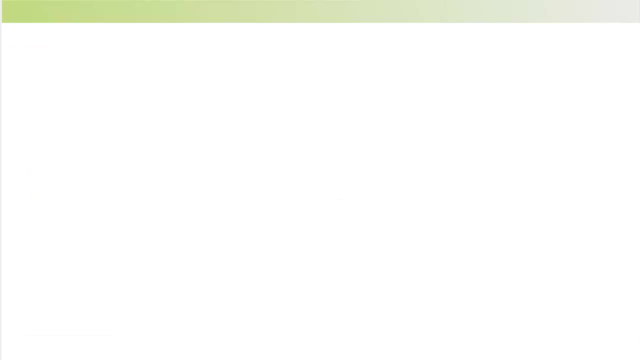 The columns may be viewed in any required order. Converting ER model into relations. Dear learners, let us now learn how entity relationship model is converted into database tables or relations. The entity relationship model is a primary source of designing database tables. If entity relationship model is modeled correctly, the database design will be perfect. 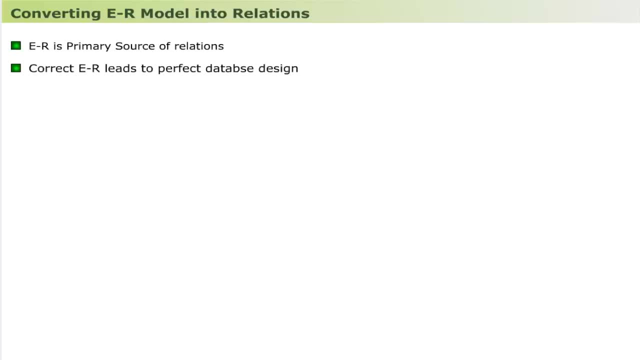 Many case tools are available to design tables from ER model. However, it is important to know the conversion mechanism of ER model into set of tables. Let us now discuss it in detail. Dear learners, remember this general rule: in order to convert an ER model, 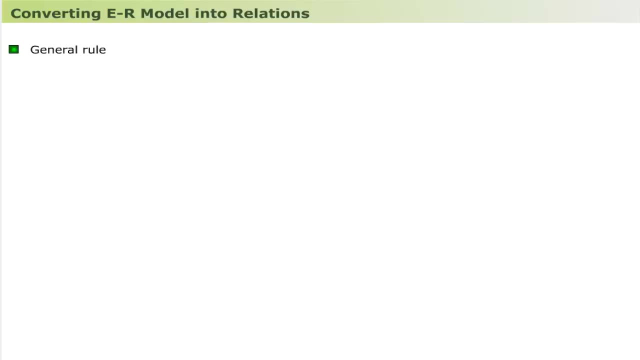 To convert an ER model into tables. the entity class is converted into a table such that: 1. Name of the table is derived from name of entity class. It is preferred that the table have same name as entity class. 2. The attributes of entity class are converted into fields or columns of the table. 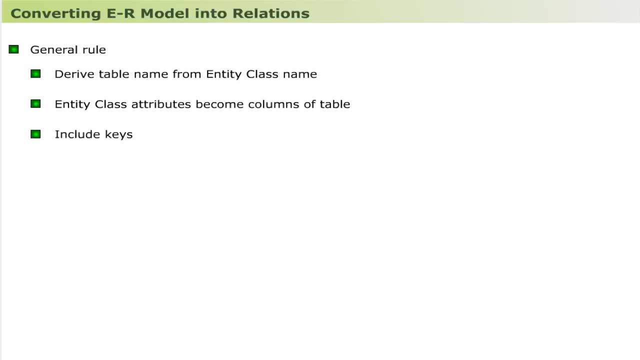 3. Include keys. Dear learners, after knowing the thumb rule of entity class conversion into table, it is now time to explore it further. Here is the detail: Regular Entity Conversion. Each regular entity class is converted into a table such that the attributes of entity class are converted into fields or columns of the table. 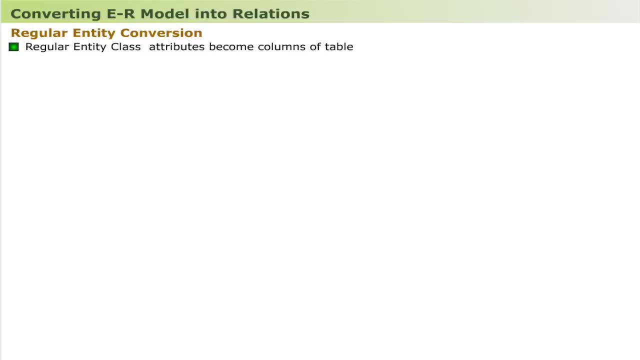 For example, let us see how the given entity class customer with attributes customer number, name and city is converted into corresponding customer table. The entity class name that is customer is converted into table name customer. The attributes of entity class customer that are customer number, name and city are converted into corresponding column names that are customer number, name and city. 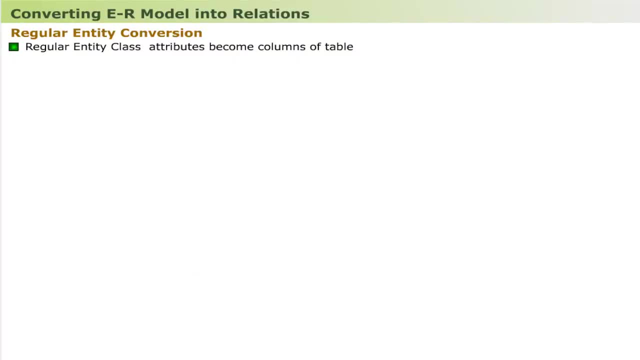 The sample rows are shown as: Let us now discuss conversion of composite attributes. If regular entity class has a composite attribute, then the atomic components of composite attributes are converted into columns, as discussed earlier. For example, Consider the entity class student- with two atomic attributes- registration number and city- and one composite attribute- name- along with constituent parts, first name and last name. 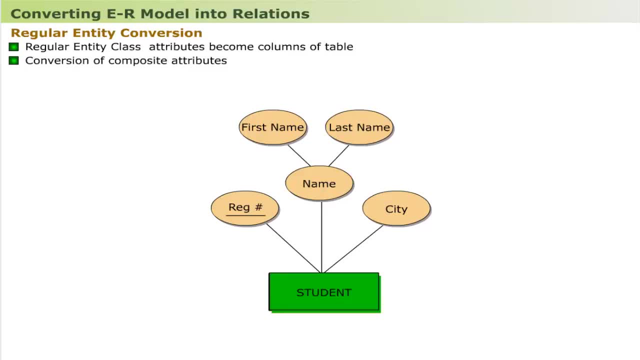 The entity class name student is converted into table name. student. The atomic attributes, registration number and city are converted into corresponding columns. registration number and city. The atomic parts of the composite attribute name that are first name and last name are converted into column names. 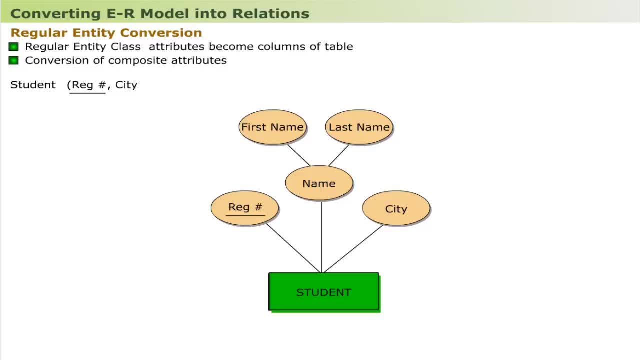 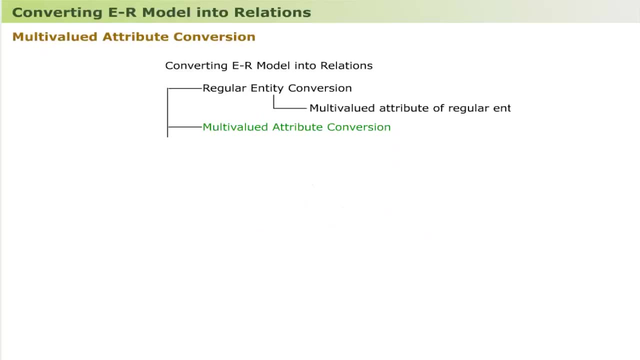 The atomic parts of the composite attribute name that are first name and last name are converted into corresponding columns: first name and last name. Multi-Valued Attributes Conversion. If regular entity class contains a multi-valued attribute, then two tables are created. The first table contains all the attributes of regular entity class except multi-valued attribute. 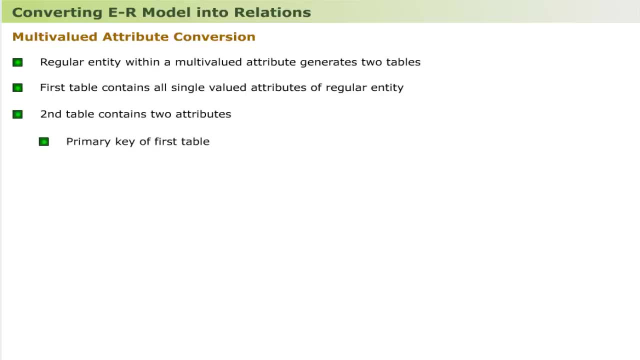 The second table contains attributes with the primary key of first table, along with multi-valued attributes of source name and last name. This table must have composite key. For example, Consider the entity class student- with two atomic attributes- registration number and name- and one multi-valued attribute- hobby. 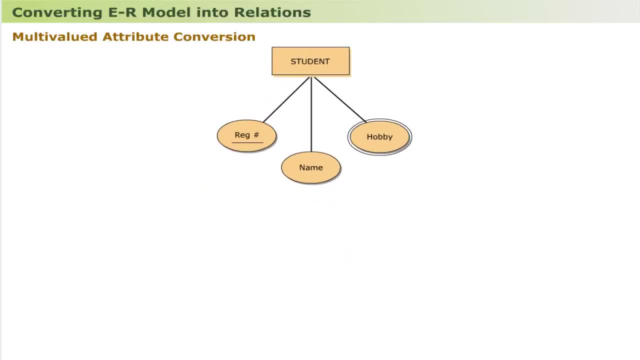 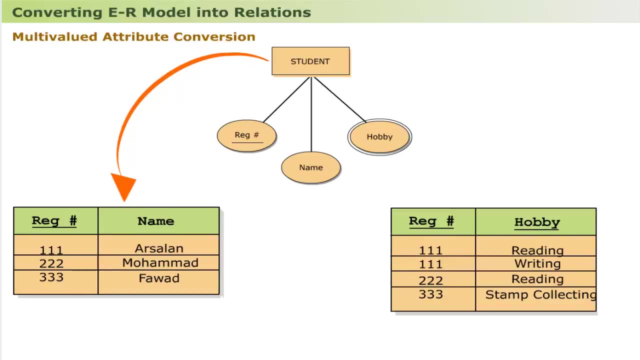 Two tables are created as shown. Number 1: The entity class name student is converted into table name student. The attributes of entity class registration number and name are converted into columns: first name and last name. The column registration number is the primary key. 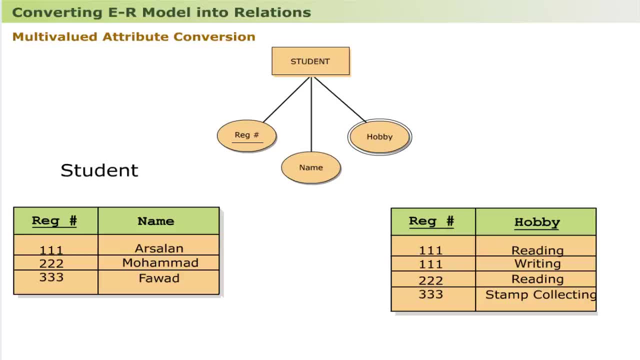 Number 2. The multi-valued attribute hobby of entity class student is converted into table name hobby. The primary key attribute and multi-valued attribute of entity class student are converted into columns of table hobby. The column registration number and hobby makes the composite key. 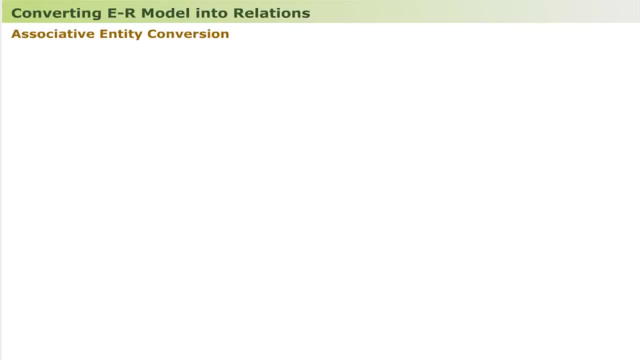 Associative Entity Conversion: If there is an associative entity, then it is converted into a table such that the primary key of regular entity is included as common attribute. The table resultant has a composite key with primary key of regular entity. For example, Consider the entity class employee with two atomic attributes: employee number and name, and the entity class skill with an attribute skill. 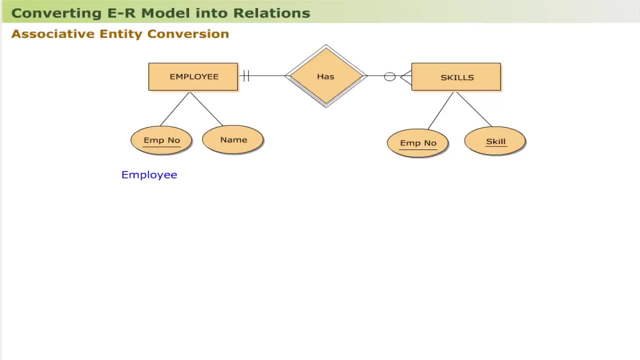 The entity class employee is converted into employee table With columns employee number as primary key name. The entity class skill is converted into skill table with columns employee number and skill with composite key. These tables are shown as The sample rows are shown as Dear learners. 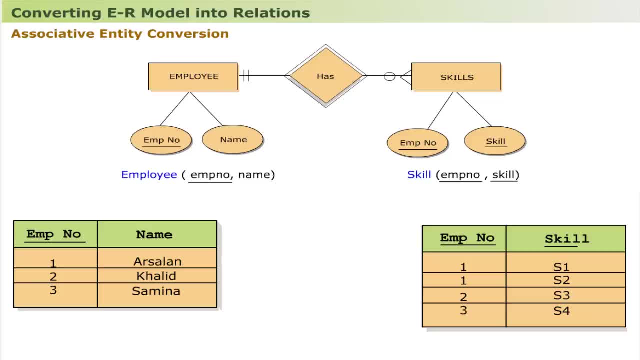 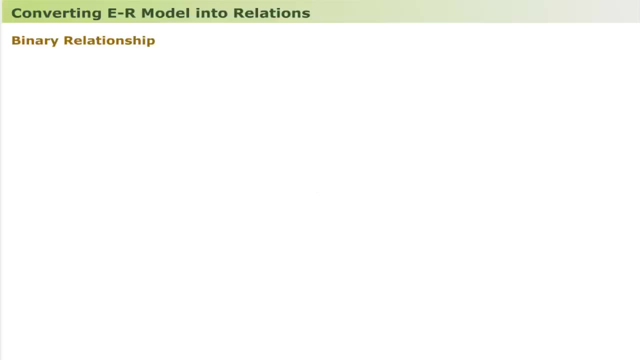 After learning conversion of various types of entity classes into tables, Now it is time to discuss How these entity classes, along with relationships, are converted into tables. Let us first discuss entity classes of binary relationship. Every entity class with the binary relationship is converted into a table. 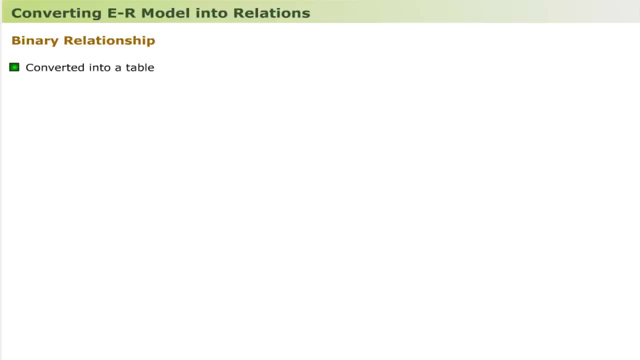 The relationship between the tables is built by defining common attribute in both the tables. Let us now discuss various types of associations involved in binary relationship. One to one association: Consider the statement that a student is allowed to register for only one project and a given project is taken by only one student. 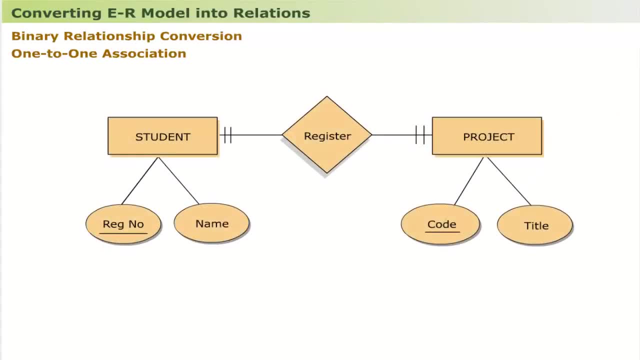 The ER model is shown as The given model is to be converted into table as Step 1. Tables formation. The entity class student is converted into student table with attributes registration number as primary key and name as shown. Similarly, entity class project is converted into project table with attributes project code as primary key and title as shown. 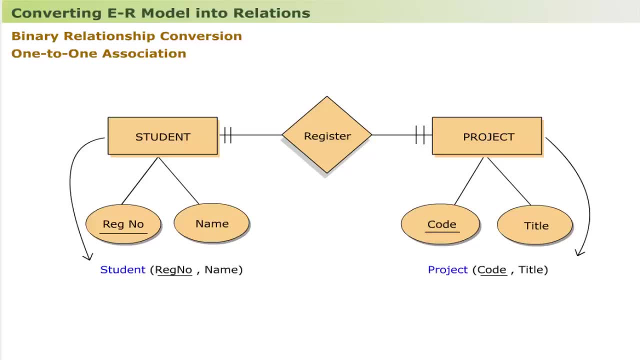 Step 2. Build relationship. The relationship between table, student and project is defined by defining common attribute in both the tables. This can be done by including the primary key of any one table in the other table as non-key attribute, called foreign key, as shown. 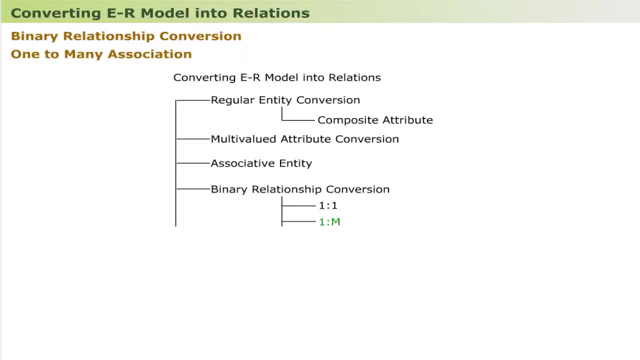 One to many association. There are two possibilities for binary one to many association. These are: 1. If the relationship has an associative entity, then each entity class is converted into a table and common attribute is already defined. Consider the ER model as shown. 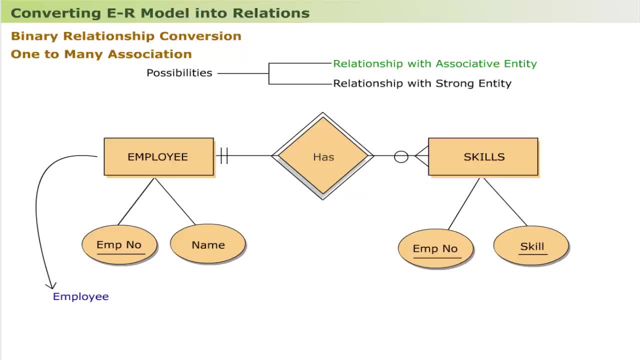 The entity class employee is converted into employee table with columns employee number as primary key and name. The entity class skill is converted into skill table with column employee number and skill both as composite key. The common attribute employee number in both the tables is already included. 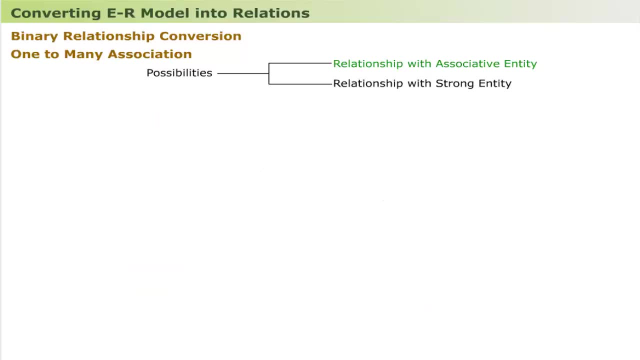 The sample rows are shown as 2.. If the relationship has strong entities, then each entity class is to be converted into a table. The primary key of table which is formed from entity class having cardinality one is to be included to the table which is formed from entity class having many cardinality as foreign key. 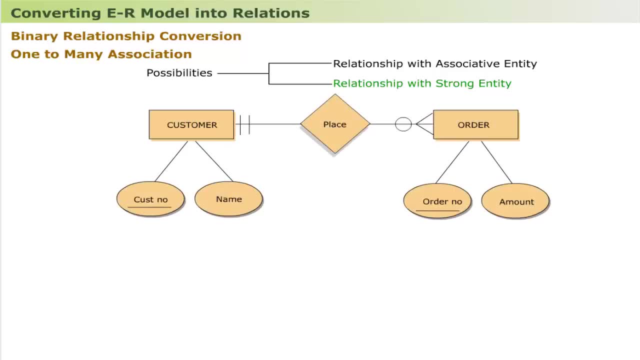 Consider the ER model. as shown, The relationship place is a binary relationship, as its degree is 2.. The entity classes are Customer, with attributes customer number as primary key, and name Order, with attributes order number as primary key and amount. Dear learners, let us see how this conversion takes place. 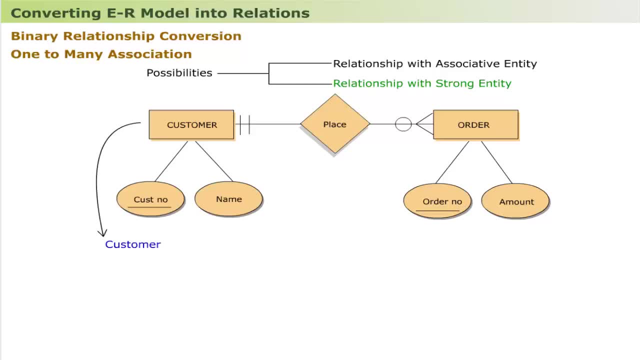 The entity class customer is converted into customer table with columns customer number as primary key and name. The entity class order is converted into order table with columns order number as primary key and amount. The relationship between these tables is formed by including the primary key of customer table, that is, attribute customer number, to table order as foreign key. 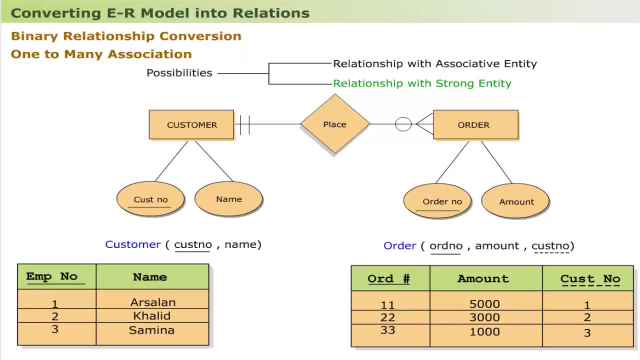 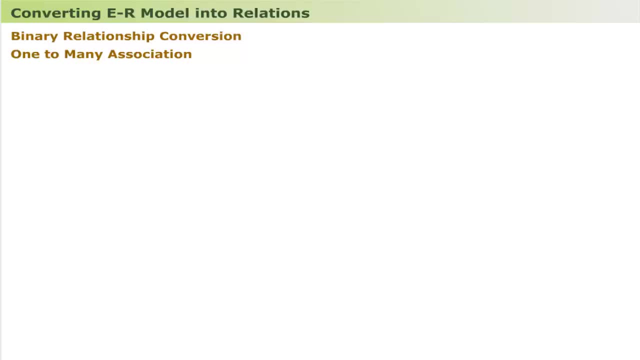 The sample rows are shown as Dear learners. So far we have discussed two types of associations of binary relationship conversion into set of tables. Now we will discuss many to many relationship conversion. Here is the detail. There are two possibilities for existence of binary many to many relationship. 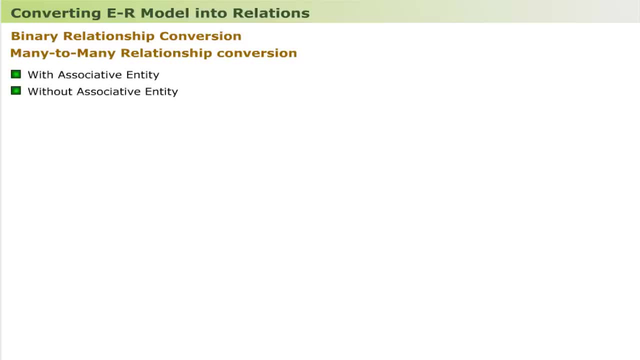 These are With associative entity, Without associative entity. Let us discuss each one in detail. With associative entity: If there is binary relationship with an associative entity, then every entity class, including associative entity, is converted into a table. The attributes of each entity class becomes columns of corresponding table. 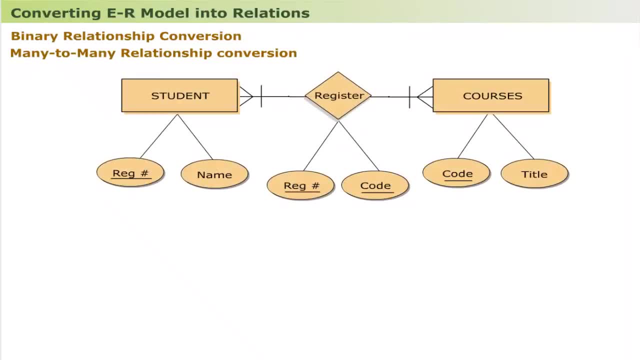 Consider the ER model as shown. Let us examine how this model is converted into set of tables. The entity class student is converted into student table with columns registration number as primary key and name. The entity class course is converted into set of tables. The entity class student is converted into course table with columns course code as primary key and title. 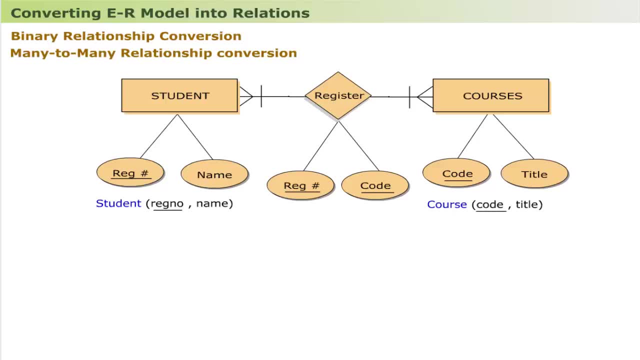 The associative entity class register is converted into registration table with columns, registration number and course code both as composite key. The sample rows are shown as Without associative entity. If there is a binary many to many relationship without associative entity, then each entity class is converted into a table. 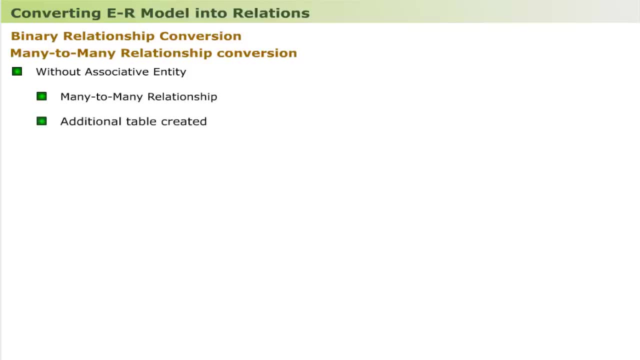 Additionally, an additional table is also created. The primary key of each table created is included in the additional table as composite key. Consider the ER model as shown. Let us examine how this model is converted into tables. The entity class student is converted into student table. 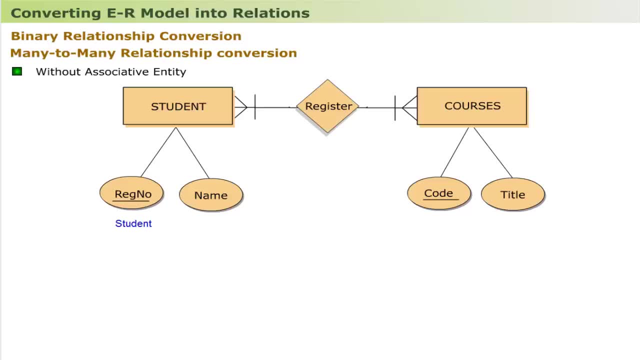 The attributes of entity class student are converted into columns of student table. The column registration number is selected as primary key. The entity class course is converted into course table. The attributes of entity class course are converted into columns of course table. The column course code is selected as primary key. 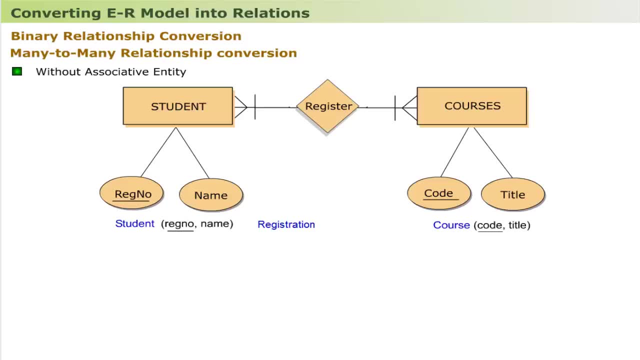 An additional table, registration, is created. The primary key of student table, that is registration number, and primary key of course table, that is course code, are included as composite key. The sample rows of student table are shown as: The sample rows of course table are shown as: 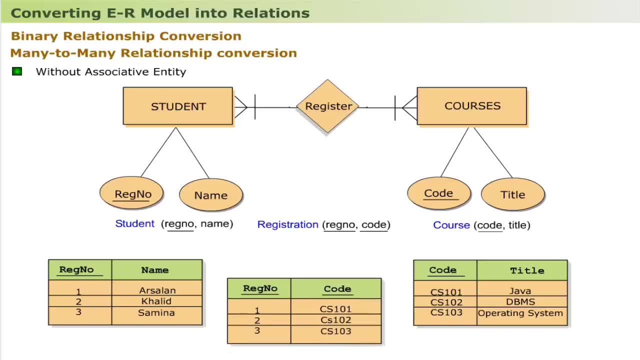 The sample rows of registration table are shown as The binary many to many relationship may also have non-key attributes, such as attribute date of registration, as shown. The table formation process is same as discussed earlier. as shown, The non-key attributes of the relationship are included in the additional table, such as date of registration in this case. as shown. 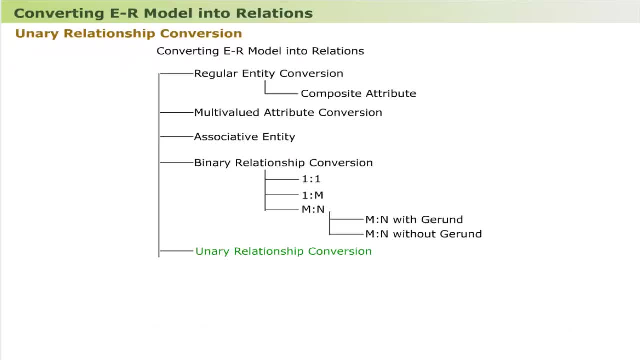 Unary relationship conversion. The entities with unary relationship are also converted into tables, just like the entities with binary relationship. The common attribute, that is, foreign key, is to be added such that it references the primary key value of the same table. Such type of foreign key is called recursive foreign key. 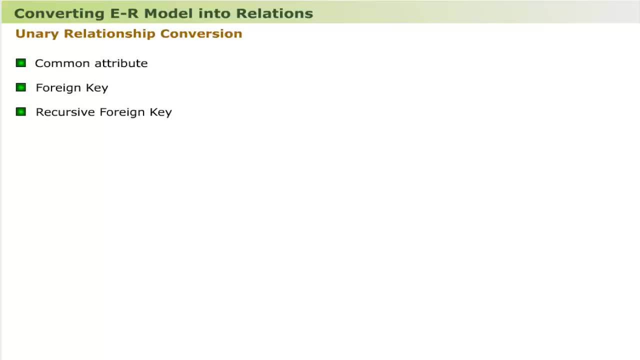 Dear learners, let us discuss various possible cases of unary relationship. These are: One to one association. One to many association. Many to many association. Here is the detail of each case: One to one association. The entity class of unary relationship of the type one to one is converted into a table. 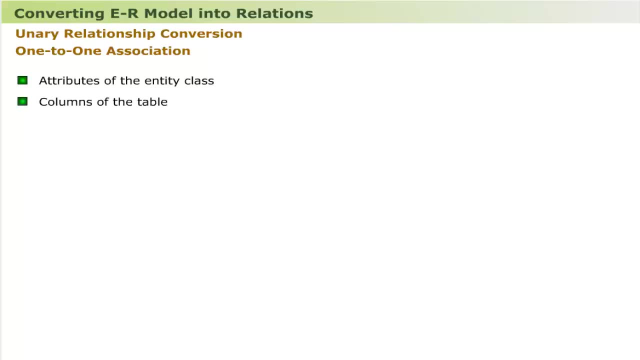 The attributes of the entity class are converted into columns of the table. The primary key of the entity class is converted into primary key of the table. This primary key is added as recursive foreign key with a new name. Consider the unary relationship manage of the type one to one with an entity class employee, as shown. 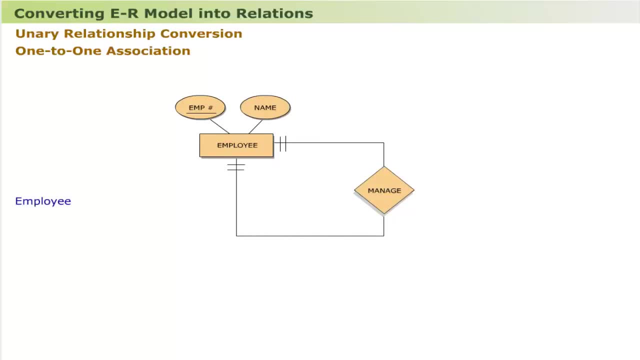 The entity class employee is converted into employee table. The attributes of the employee- employee number and name- are converted into columns of the table. The primary key of the entity class employee is converted into primary key of the table- employee. This primary key is added as recursive foreign key with a new name: manager. 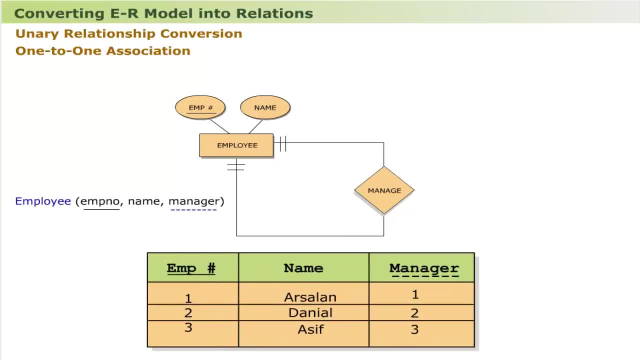 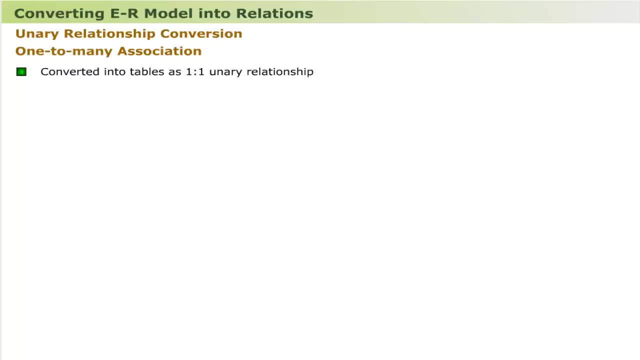 The sample rows of employee table are shown as: One to many association. The one to many unary relationship is converted into tables in the same manner as one to one unary relationship, as discussed earlier. Many to many association, The entity class of unary relationship of the type many to many is converted into two tables. 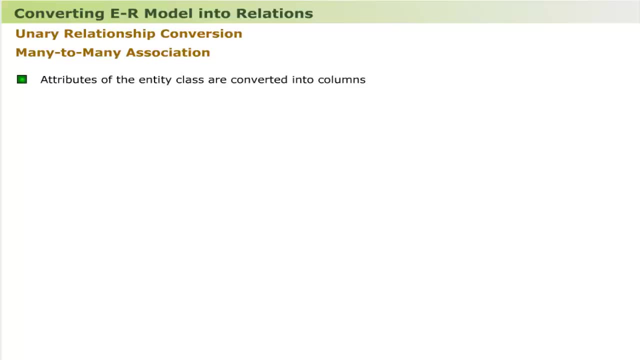 The attributes of the entity class are converted into columns of one table. The primary key of the entity class is converted into primary key of the table. An additional table is also created. The primary key of the table created from entity class is included in the additional table along with another column which is: 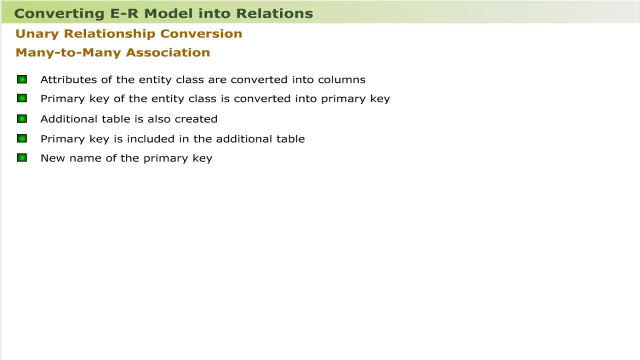 with a new name of the primary key of the same table. This additional table must have composite key. Consider the unary relationship manage of the type many to many with an entity class employee as shown, The entity class employee is converted into employee table. The attributes of the employee class, employee number and name are converted into columns of the table. 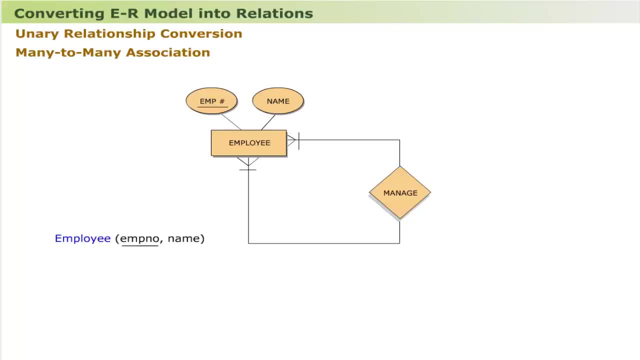 The primary key of the entity class employee is converted into primary key of the table employee. An additional table manager is created. The columns include the primary key of employee table and an additional column manager. The columns employee number and manager forms the composite key. 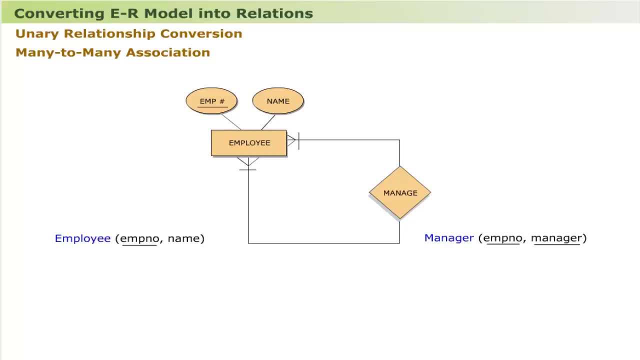 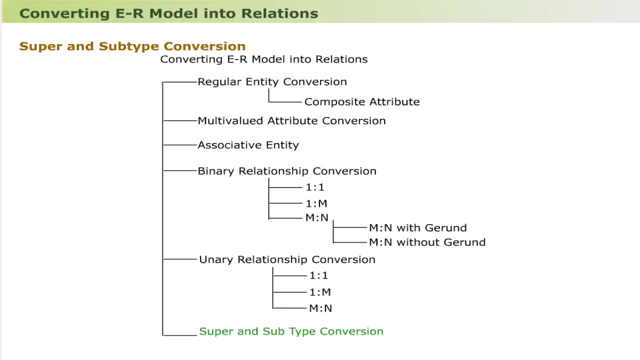 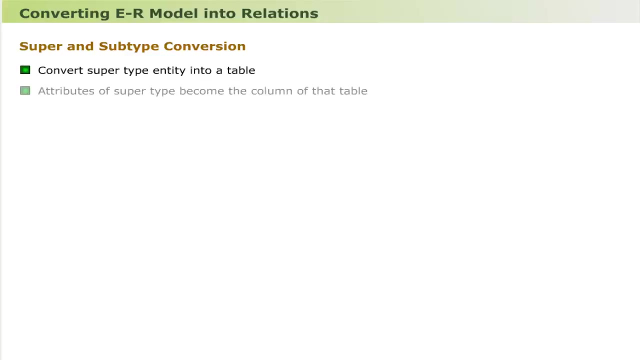 This primary key is added as recursive foreign key with a new name: manager. Super and subtype conversion. The super and subtype relationships are converted into tables. as Convert supertype entity into a table, All the attributes of supertype become the column of that table. The key of supertype will be the key of resultant table. 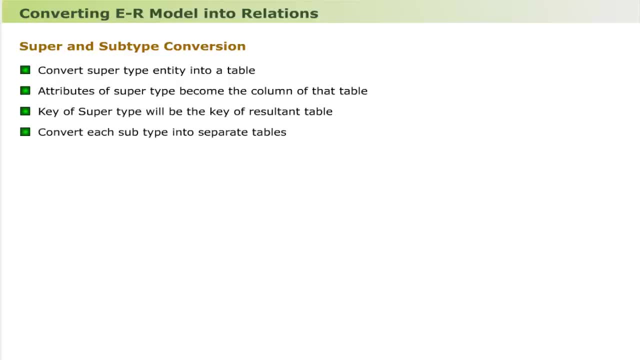 Convert each subtype into separate table. The attributes of all subtypes will become the columns of respective tables. The key of supertype table will be included into all tables. Consider the super and subtype ER model as shown. Dear learners, let us examine how this model is converted into tables. 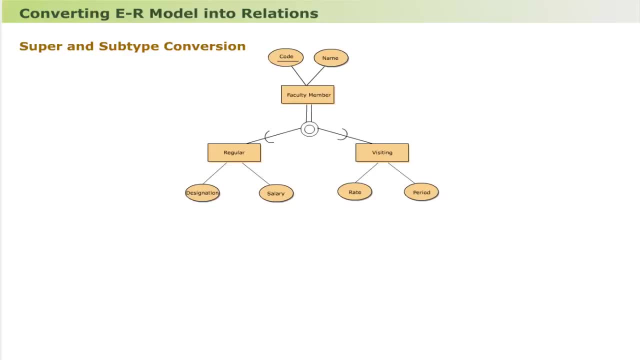 Here is the detail: The supertype entity faculty member is converted into faculty table with columns employee code as primary key and name. The subtype regular is converted into regular table with columns employee code as primary key, designation and salary. Similarly, the subtype visiting is converted into visiting table with columns employee code as primary key, rate per hour and contract period. 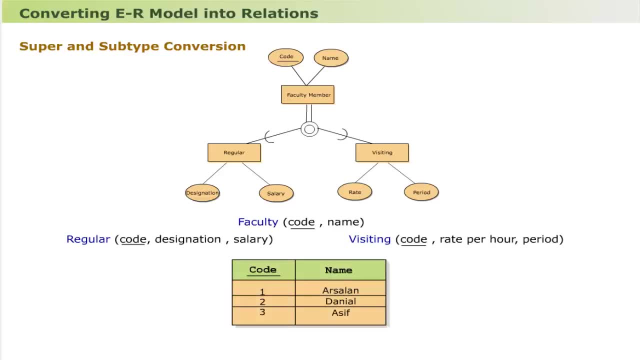 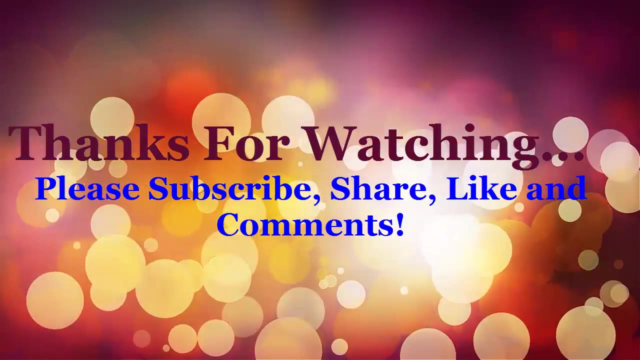 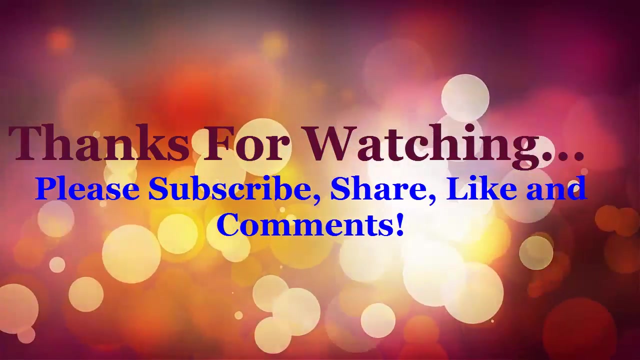 The sample rows of faculty table are shown as The sample rows of regular table are shown as The sample rows of visiting table are shown as The sample rows of lecture holds are shown as The sample rows of high elder tables are shown as: Here is the student. Already. you see, the subtype is prefixed with column employees code. Let's complete the simple superpower simulation. All equipment stunned. 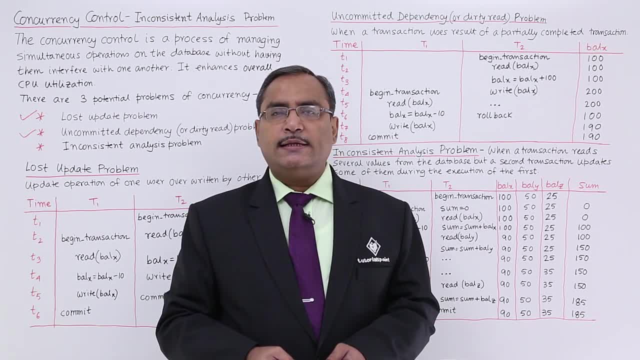 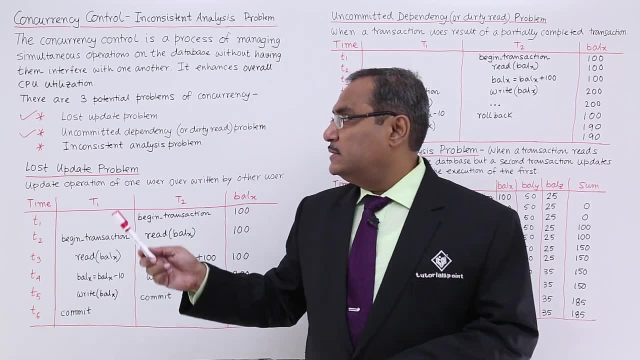 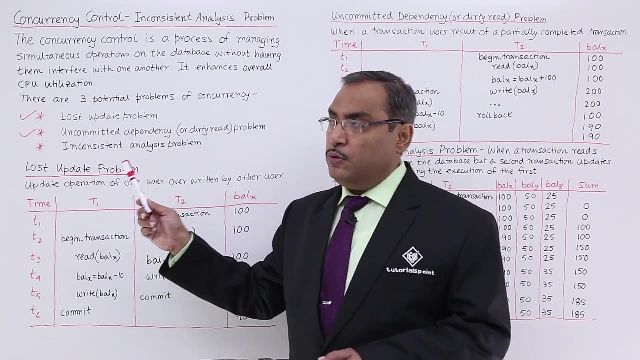 In this session we are discussing the third category of problem, that is, the inconsistent analysis problem. In the earlier videos we have discussed concurrency control. We have discussed the category one problem, that is, the lost update problem, with the proper example. We have discussed uncommitted dependency problem with one proper example: uncommitted dependency. 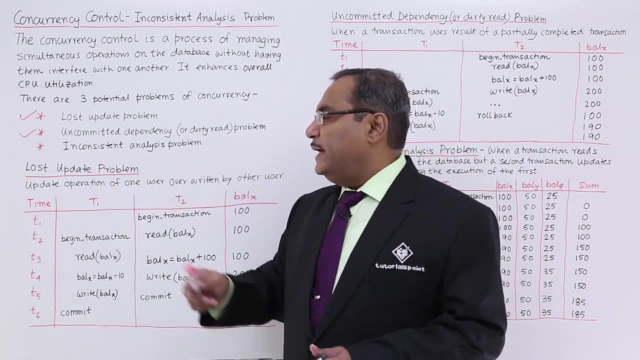 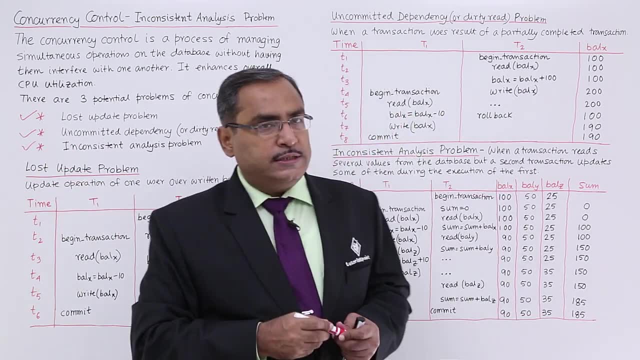 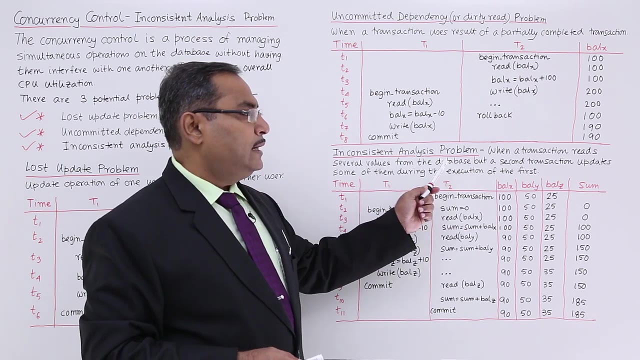 problem. Now in this video we are going to discuss inconsistent analysis problem. Please watch previous videos to have a continuation Now. inconsistent analysis problem. See, this is the problem When a transaction reads several values from the database but a second transaction updates some of them during the execution. 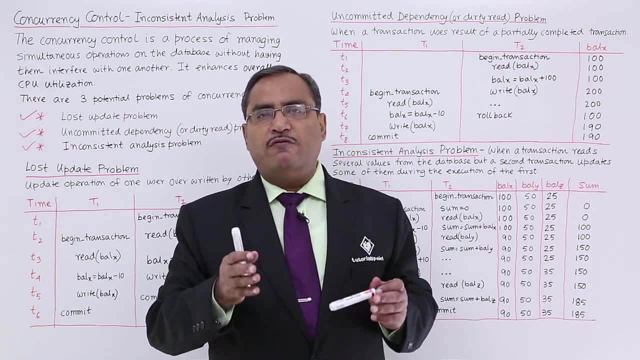 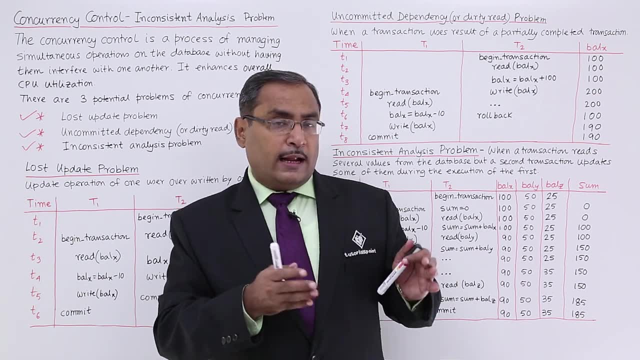 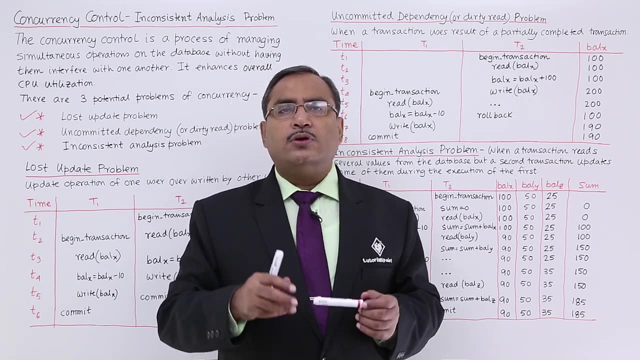 of the first, One transaction is doing some processing with the values of some variables fetched from the database And concurrently another transaction is doing some updating on that some outdated and native categories And they are now giving some updates on those values. So that is known as the inconsistent analysis problem. 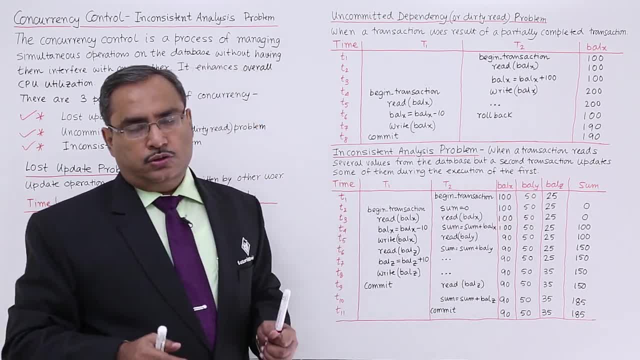 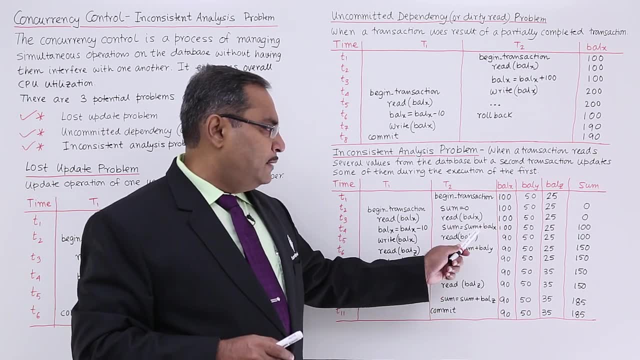 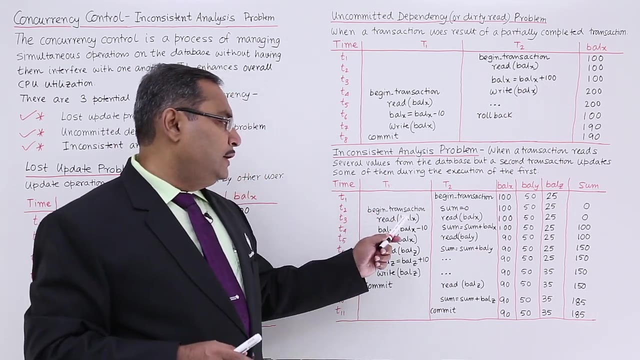 So let me give you one example for that. Here we are having three variables: balance x, balance y and balance z, So they will be rated from the database, And another variable, sum. This transaction T 2 is having a purpose to add balance x, balance y and balance n.